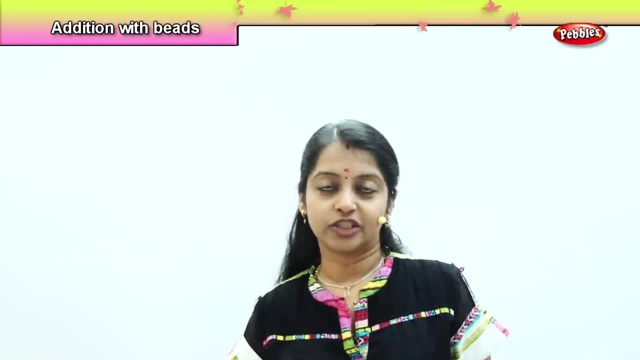 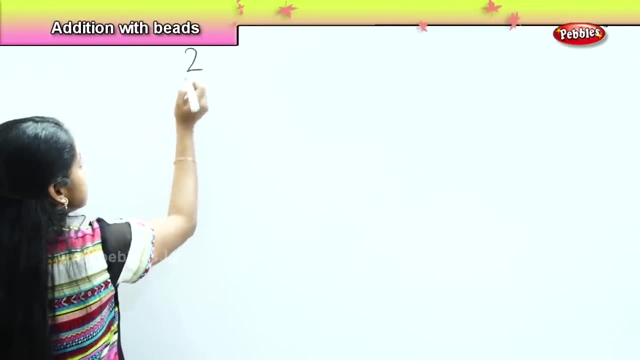 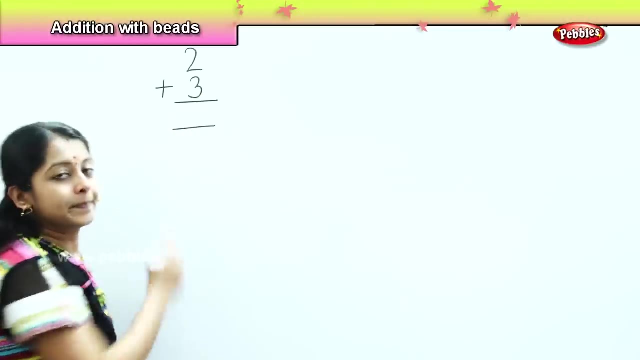 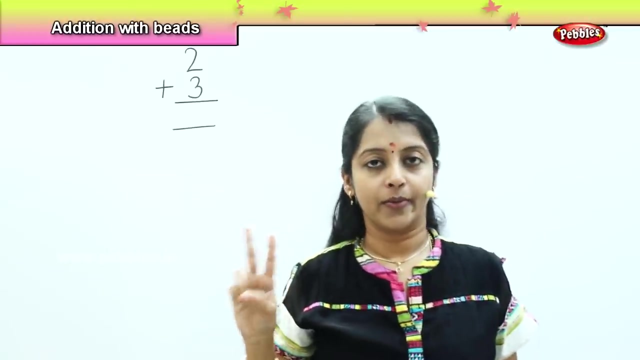 your fingers while doing the addition. So shall we begin? Okay, fine, So here now I will give you an example. What number is this? It is number 2.. And what number is this? It is number 3.. So now I have 2 fingers in my right hand, right, And I take 3 in my left hand. 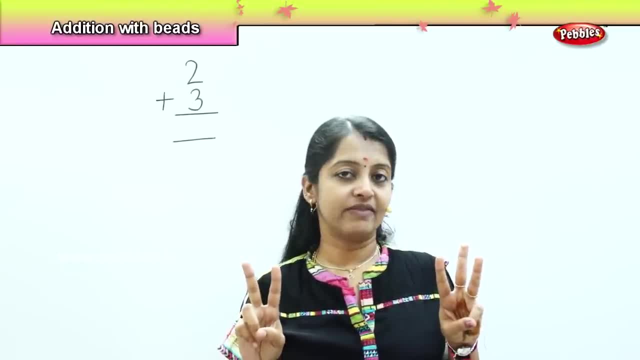 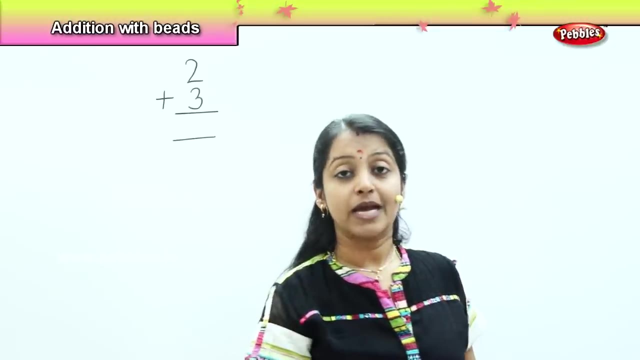 So how many fingers do I have in total? Shall we count 1,, 2,, 3,, 4 and 5.. So how many fingers do I have in total? I have 5 fingers in total. So what is my? 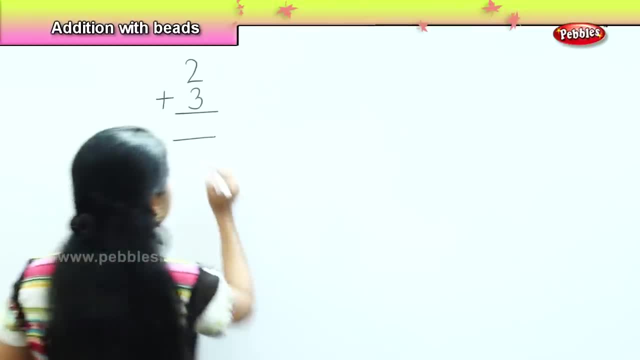 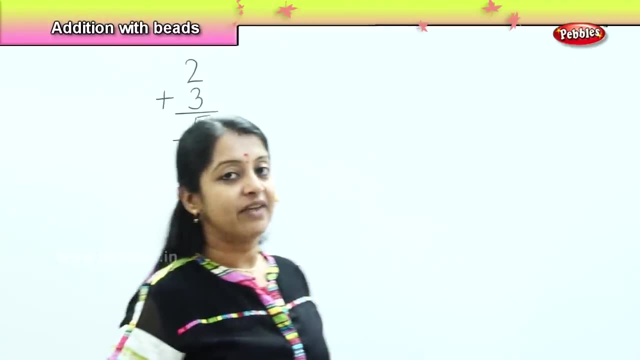 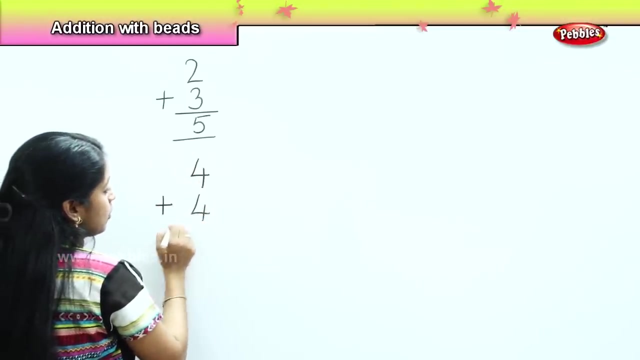 answer. My answer is 5.. Is it simple to use children? Yes, Shall we do with one more example? Yes, So what number is this? 4. See, I am putting 4 fingers in my hand right, So I have two fingers in my left hand right. 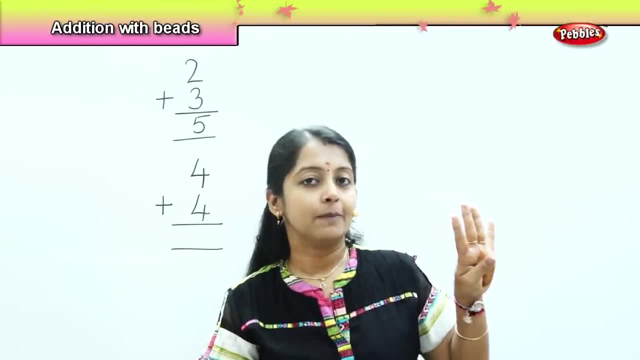 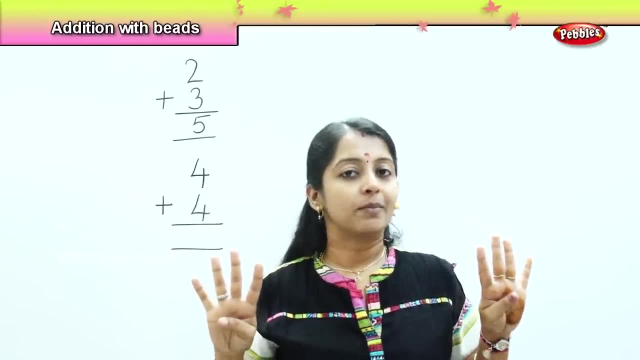 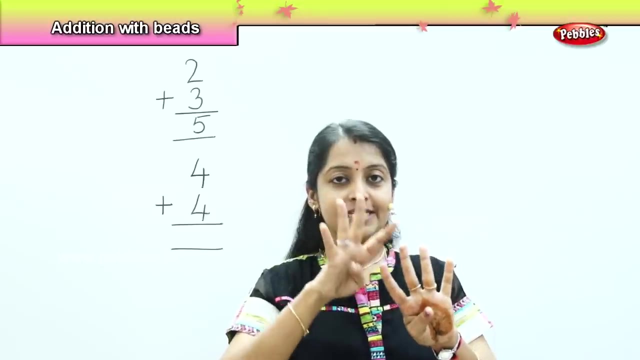 So how many fingers do we have in total? 6 fingers in each hand. What number of fingers do I have to beat 7 fingers, right? So my answer is 7 in the first number. So I need to take 4 in 1 hand and 4 in another hand. So now I have 4 fingers in my left hand and I take 4 fingers in my right hand. Shall I add the totem number of fingers, It is 1, 2,, 3, 4,, 5,, 6,, 7, 8.. So how many fingers do I have in total? Very, 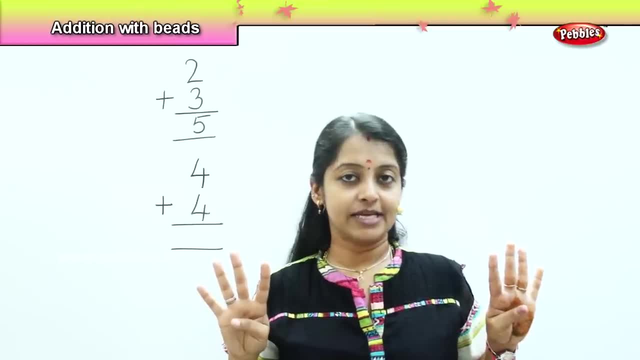 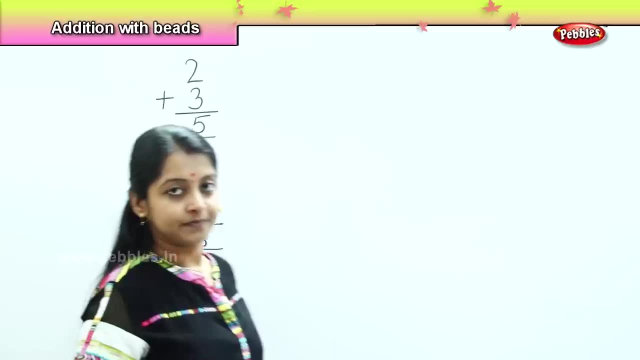 good: 1,, 2,, 3,, 4,, 5,, 6,, 7,, 8.. So how many fingers do I have in total? Very good, Very good, I have 8 fingers in total. So what will be my answer? My answer will be 8.. Right, 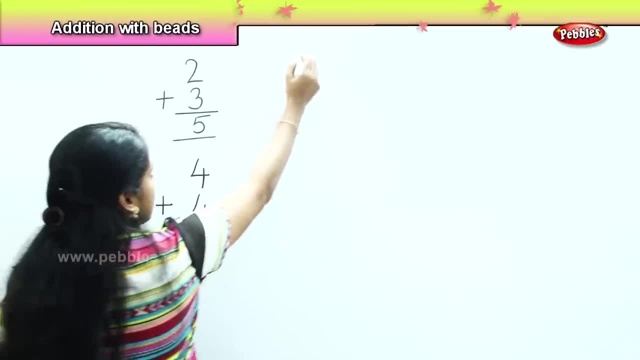 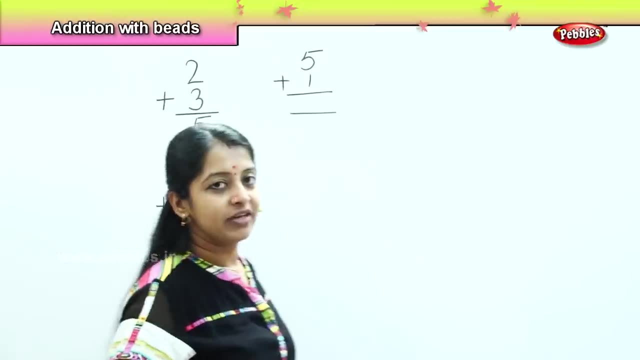 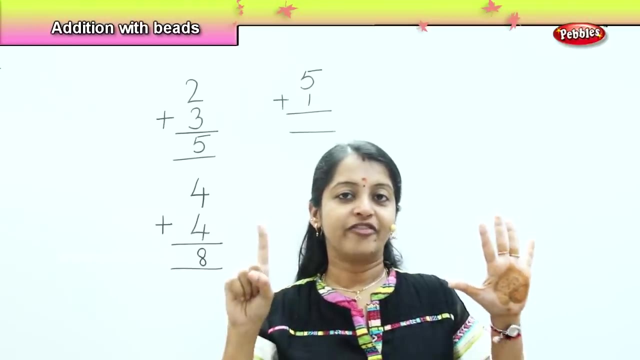 Shall I give you one more sum, No 5 plus 1.. So how many fingers you need to take in your first hand? I will take 5 fingers in one hand and 1 finger in another hand. Shall I count what is. 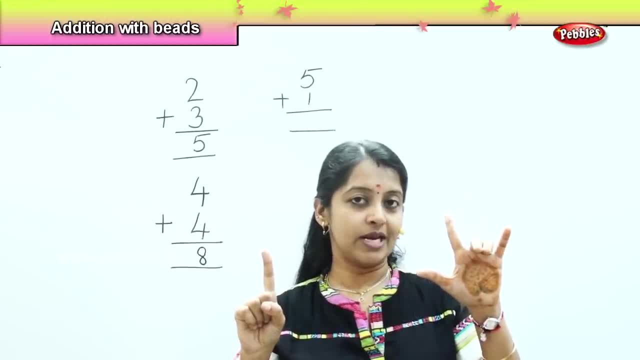 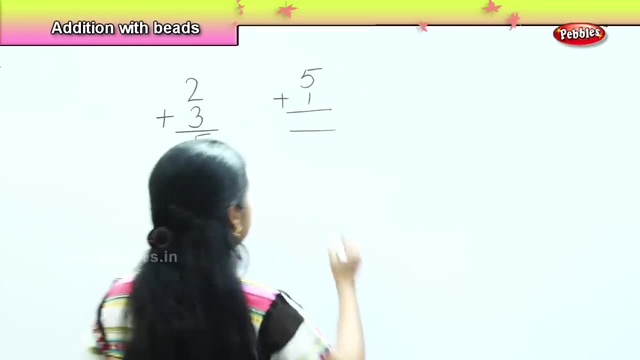 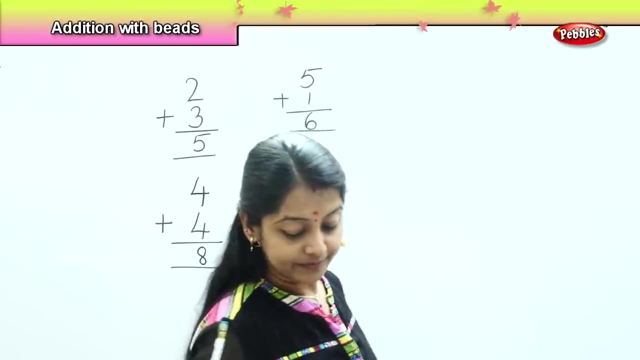 the total. It is 1,, 2,, 3,, 4,, 5 and 6.. So what is the total answer? What is the answer which I get here? It is number 6.. Okay, Now I have 2,. 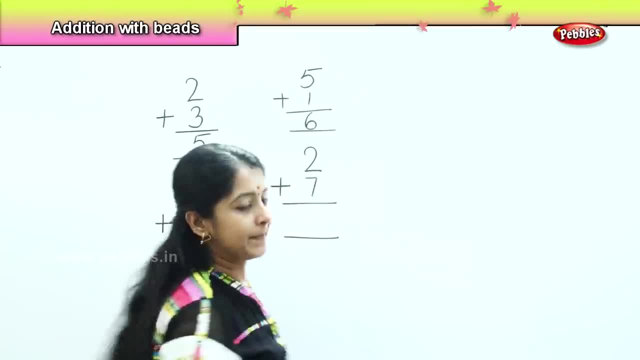 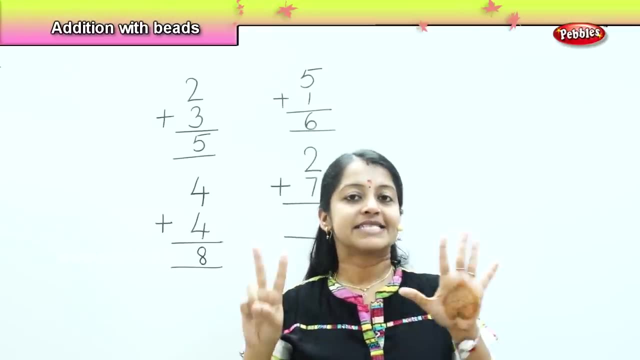 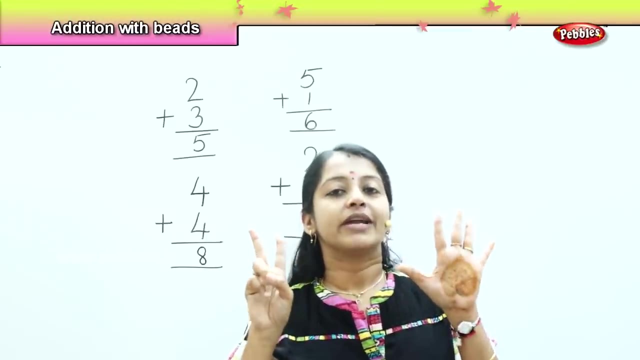 and 7.. So how will you take 2 and 7?? So first, what will I do? I will take 7 fingers together. Okay, Because we cannot have 7 fingers in one hand, Right? So I will take 7 fingers together. 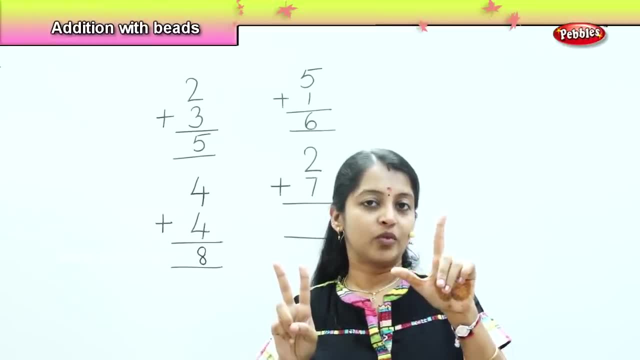 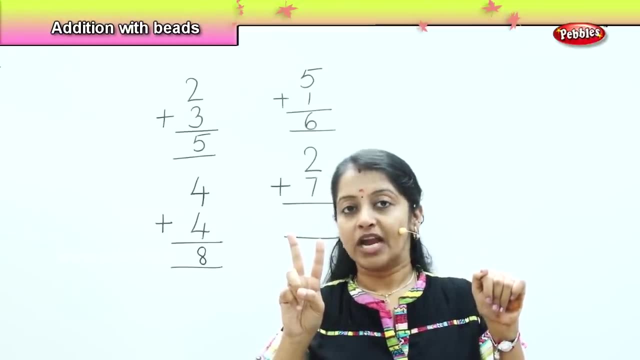 Shall, we count 1,, 2,, 3,, 4,, 5,, 6,, 7.. And what is the number which I need to add? I need to add 7 fingers, So what is the total? It is 1,, 2,, 3,, 4,, 5,, 6,, 7.. And what is the number? 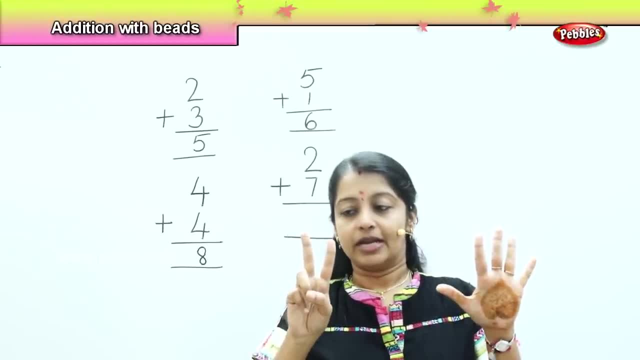 which I need to add 2 extra, Which means 7,, 8,, 9.. So what is the answer I get here, children? The answer which I get is 9.. So my answer for this question is 9.. 7 when added with 2. 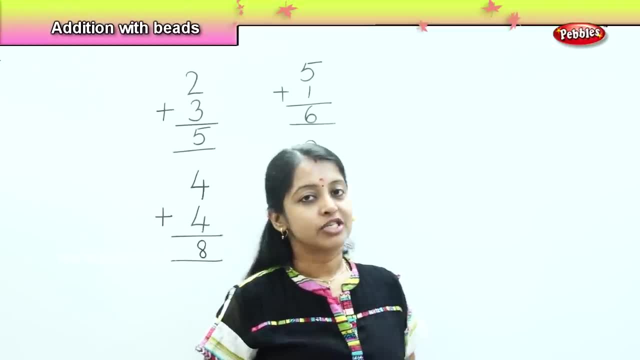 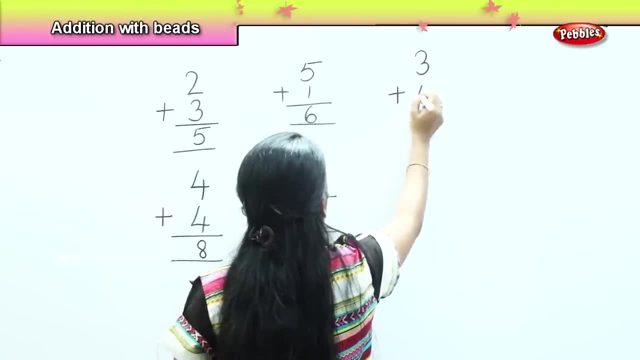 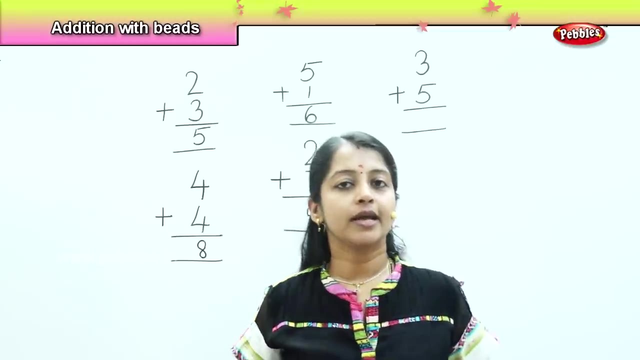 will give me an answer 9.. Okay, So shall I give you one more question Now? I have 3 and 5. So what is the answer I get here? What should I take? I should take 5 in one hand and 3 in. 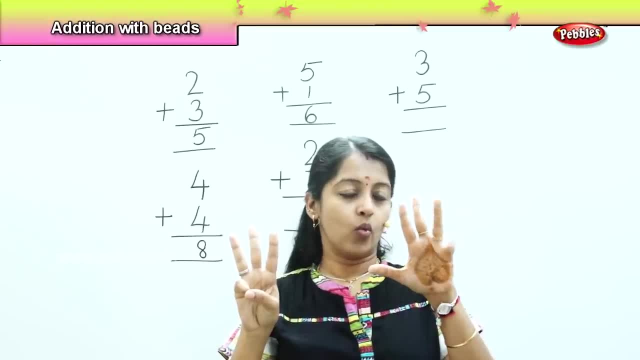 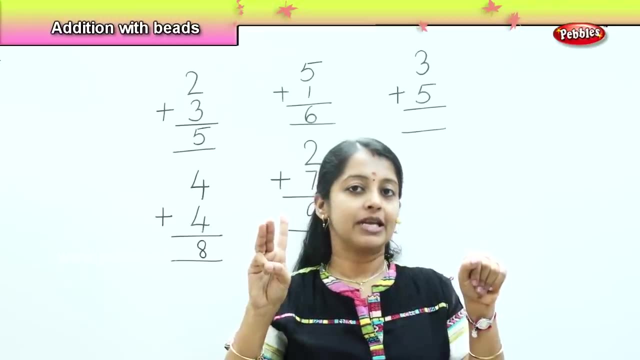 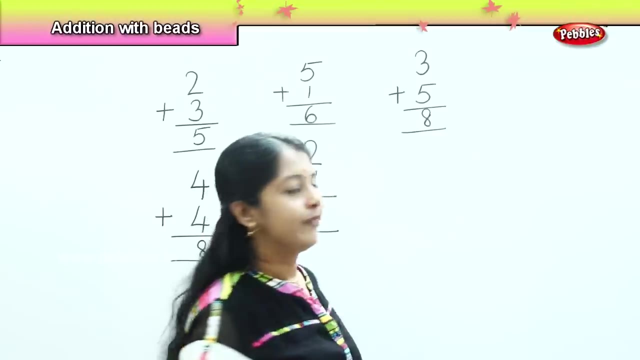 another hand. So how should I add? 1,, 2,, 3,, 4,, 5,, 6,, 7,, 8.. So what is my answer? Very good. So 3, when added with 5, will give me the answer 8.. 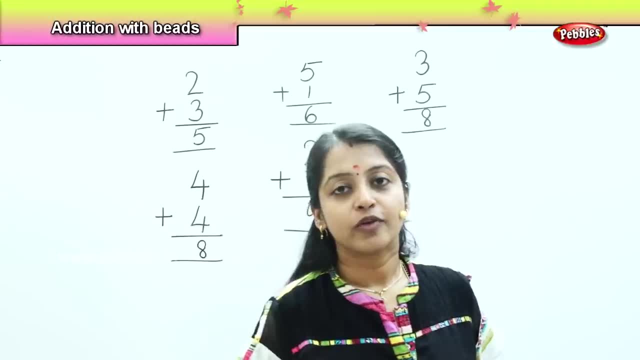 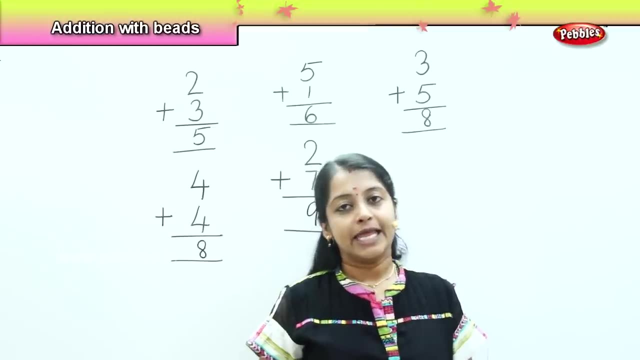 so was this method important and useful for you children? yes, you all understood this method. this is even more simpler than the previous method, which we have learned right, so i hope you enjoyed this method and again we will be doing some more practice sums to understand these better. 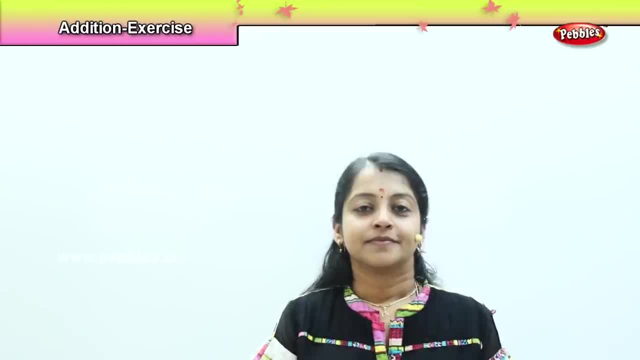 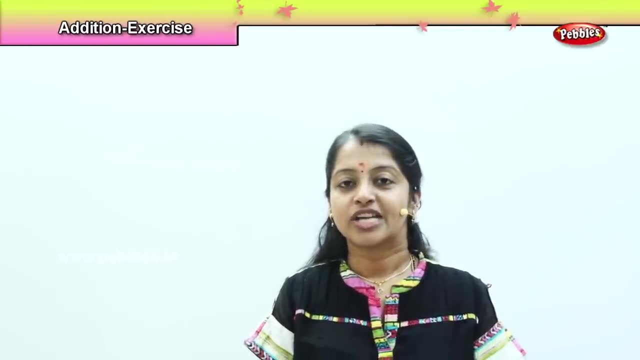 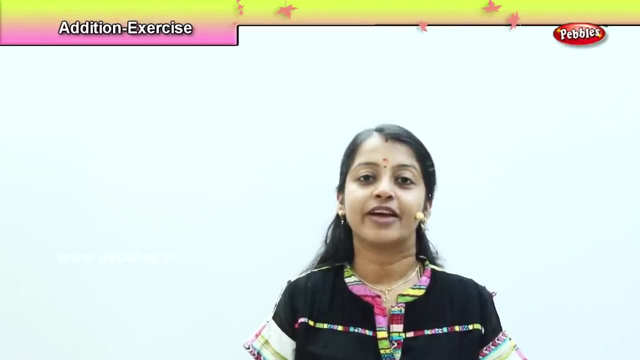 okay. so, children, we have learned quite a new stuff in addition process, so shall we do a quick recap of whatever we have learned till now? so what, what and all we learned? we learned additional facts. then we learned counting by beads, we learned counting using fingers, and we also learned how. 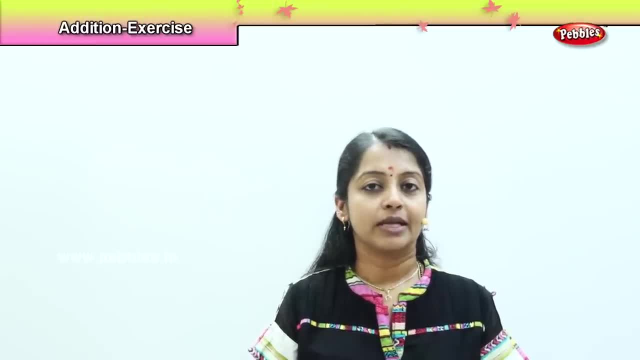 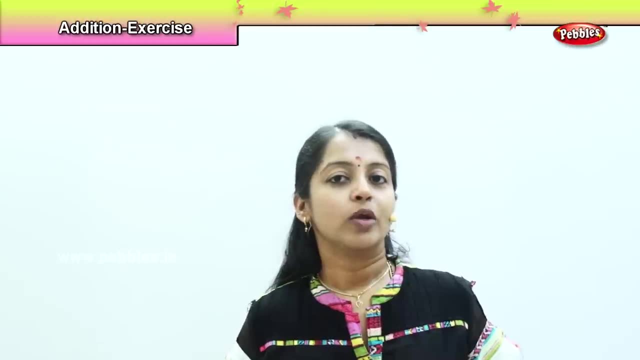 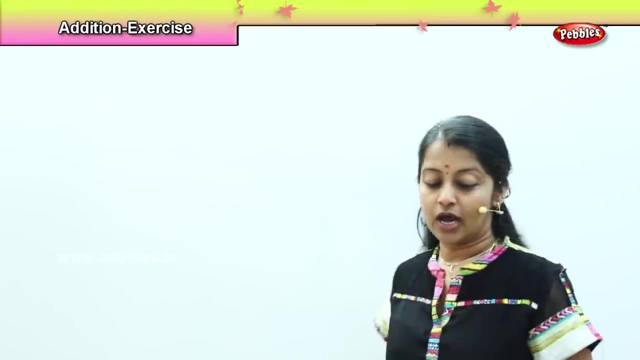 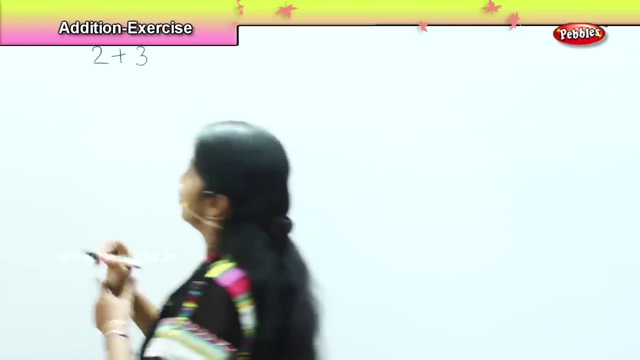 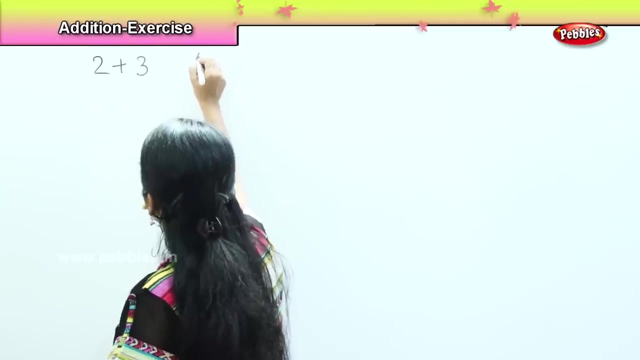 to count by drawing the pictures and counting them with the numbers, right. so now i will be giving you few exercise questions and you will be doing along with me and finding the answers. shall we do a quick recap? okay, fine. so now the very first question which i will give you is this: now, 2 plus 3 will be what. i will give you three answers. 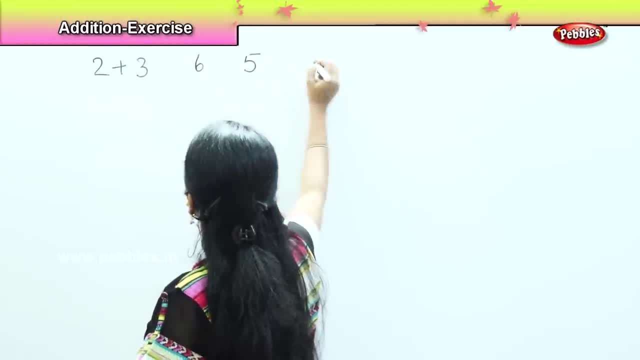 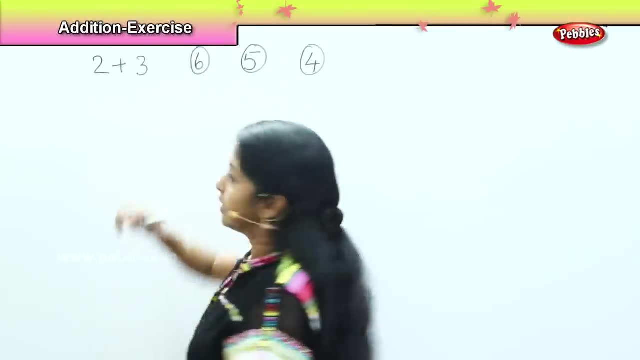 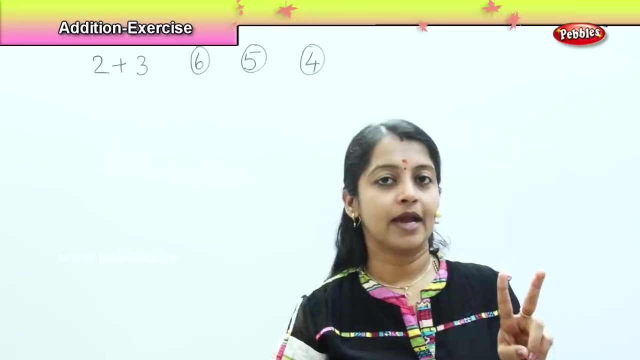 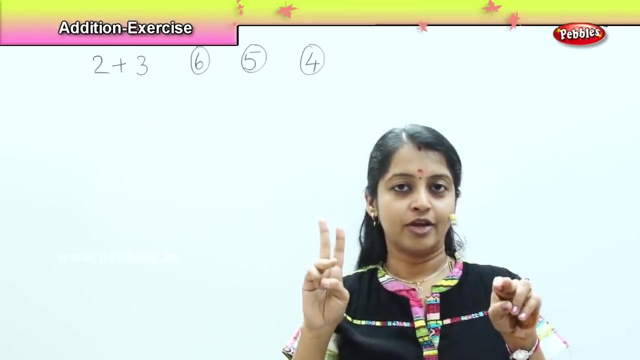 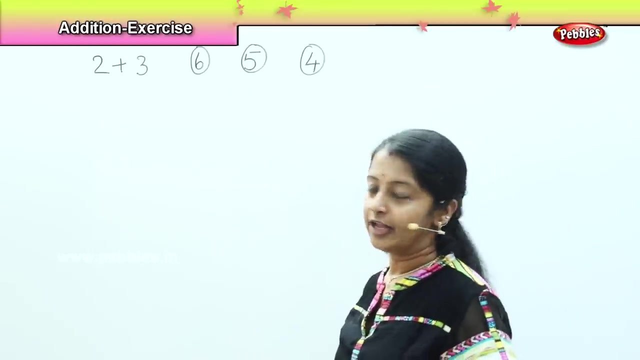 you need to select the correct answer for this. Okay, So shall we do the counting using the finger method? Okay, What you will do, You will keep 2 in one hand and 3 in another hand. So what is the total here? 1, 2,, 3,, 4 and 5.. So what is the correct answer? children, It is number 5.. 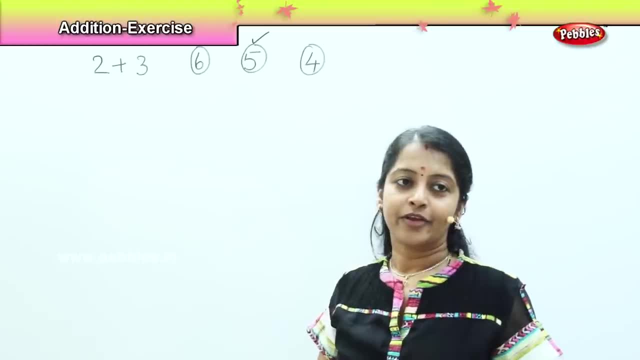 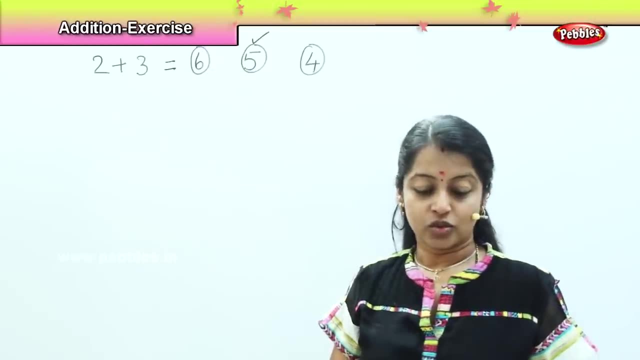 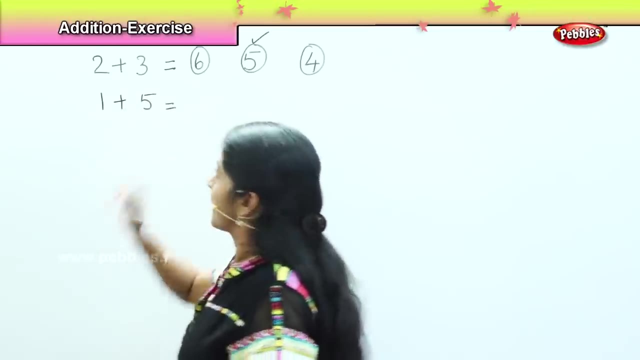 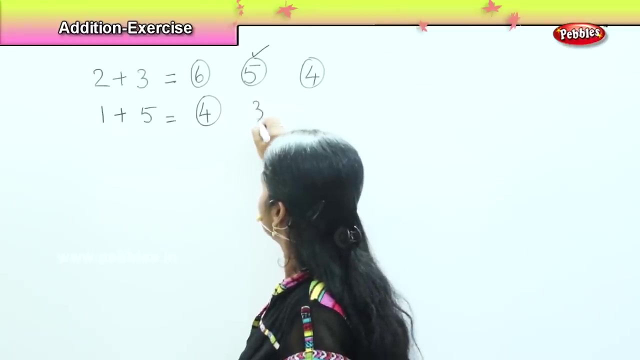 So I will put a tick on number 5.. Okay, Fine, So the next question which I will give you is 1 plus 5.. So now, 1 plus 5 will give me what answer You need to find and tell me. 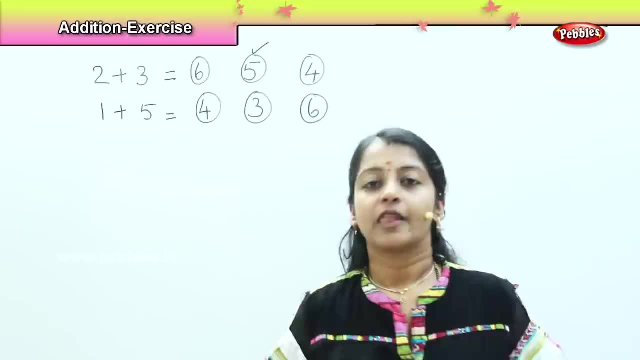 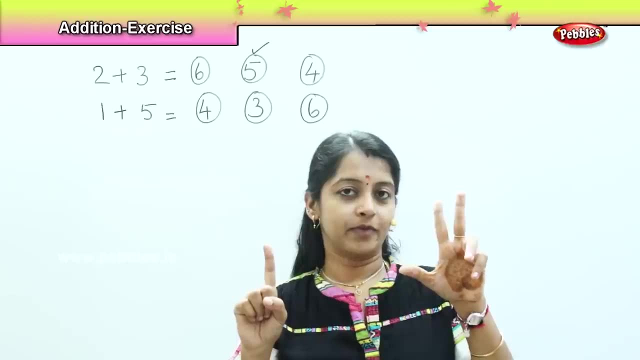 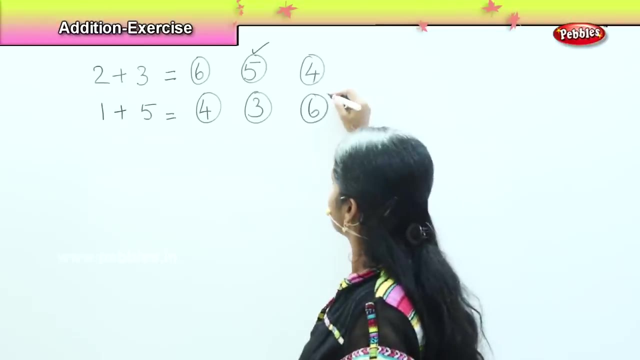 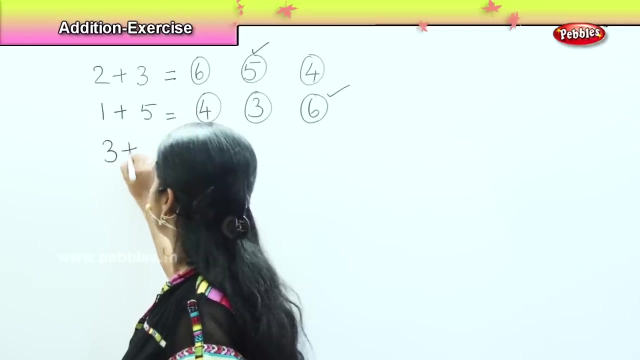 Now what will I do? I need to give 5 in one hand and 1 in another hand. Shall I count 1,, 2,, 3,, 4,, 5 and 6.. So my answer is 6.. Very good, So the next question which comes here is: 3 plus 4 is. 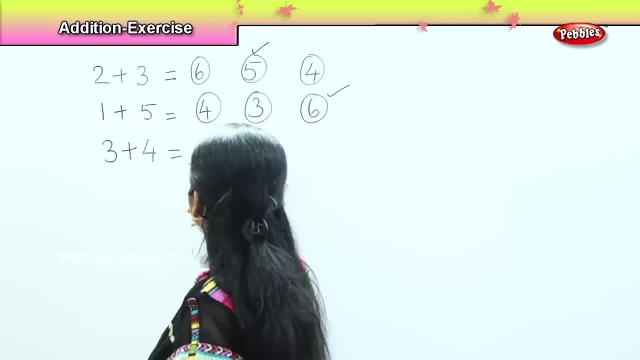 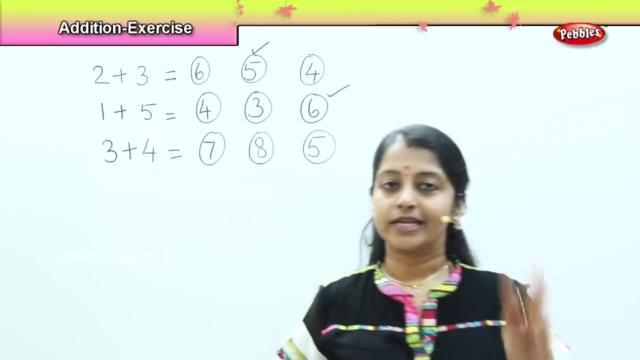 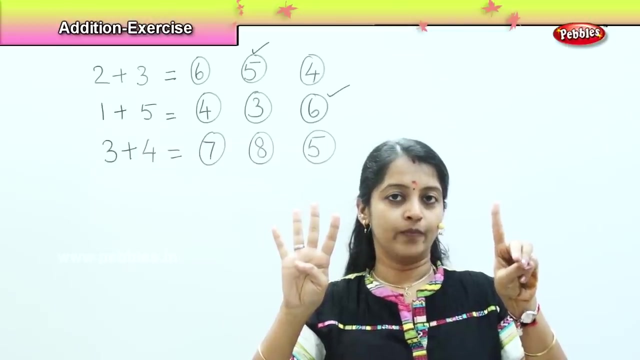 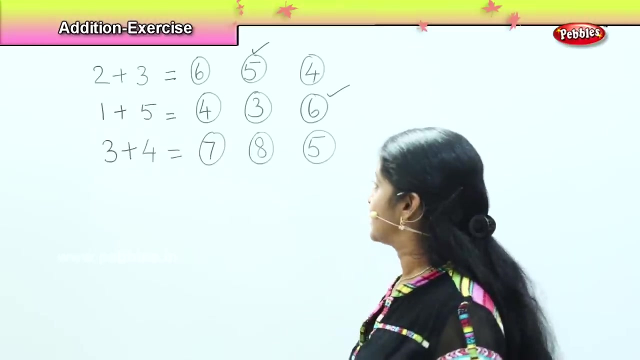 equals to what You need to find and tell me the answer. So what you will do? You will keep 3 in one hand and 4 in another hand. Shall we count 1,, 2,, 3,, 4,, 5,, 6,, 7.. So what is my answer? My answer is 7.. Fine, 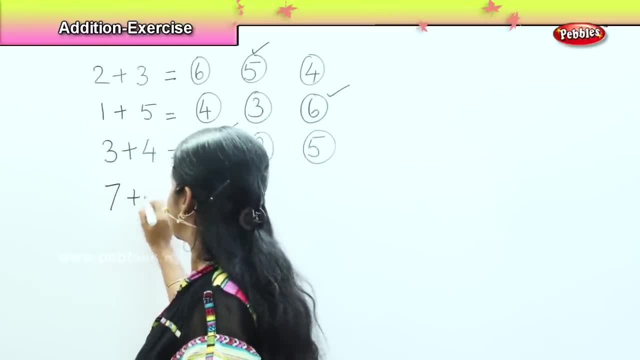 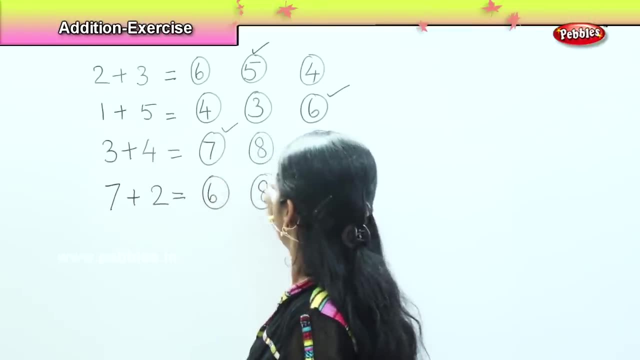 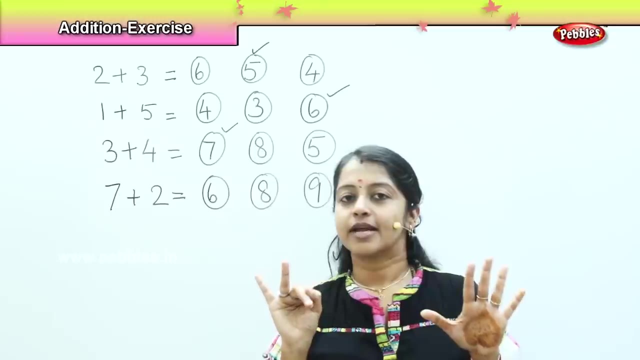 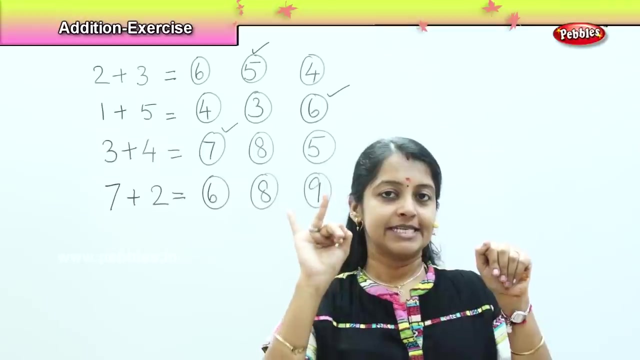 So let us come to the next question, which is 7 plus 2 is equals to what. So what I need to do, children here, I need to keep 7 fingers in together Right, So 1, 2,, 3,, 4,, 5,, 6,, 7, and add 2 extra, So 8 and 9.. 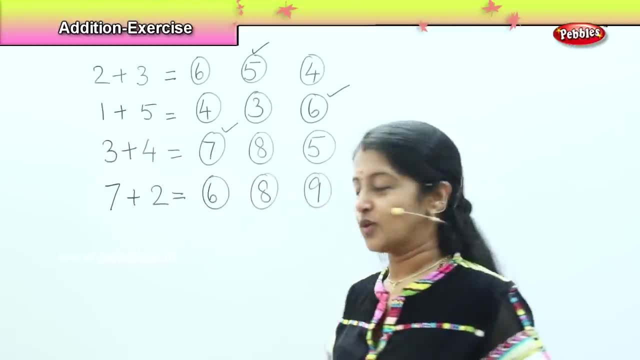 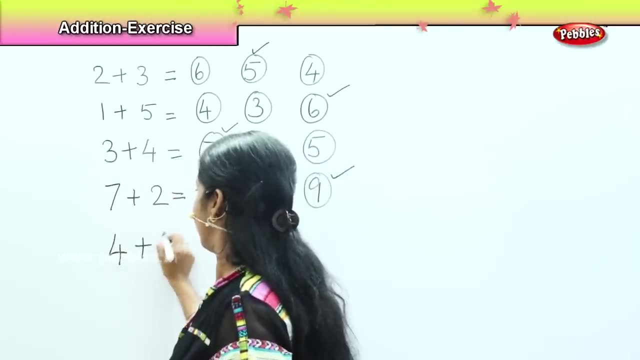 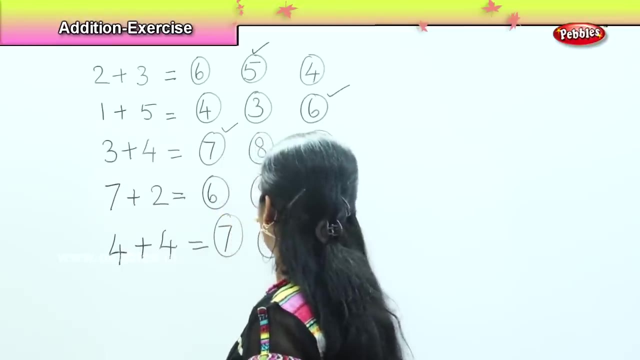 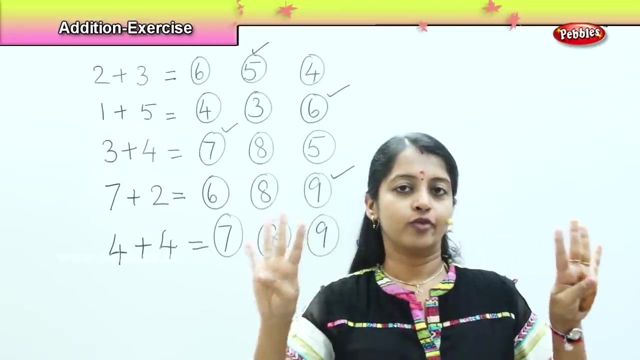 So how many fingers I have? The answer for this question? The answer for this question is 9.. Very good. The next question which comes here is: 4 plus 4 is equals to what. So here comes your answer: What you need to do, children, You need to have 4 in one hand and 4 in another hand. 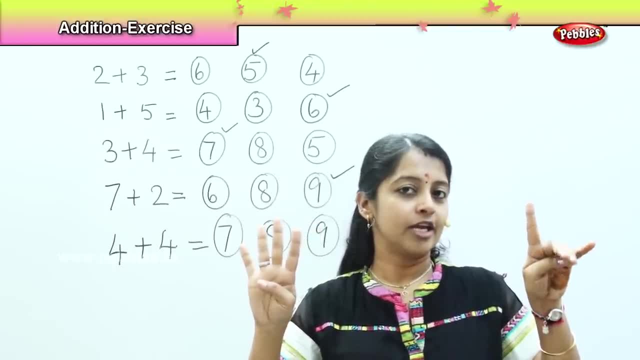 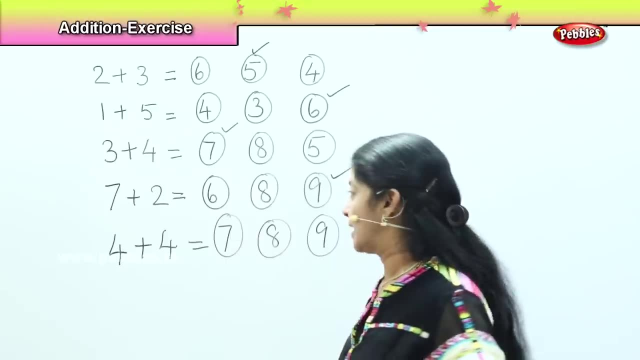 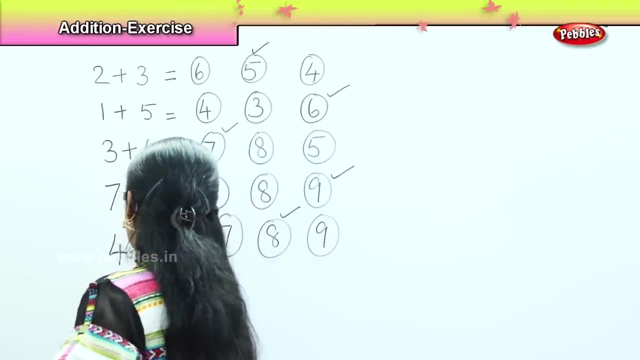 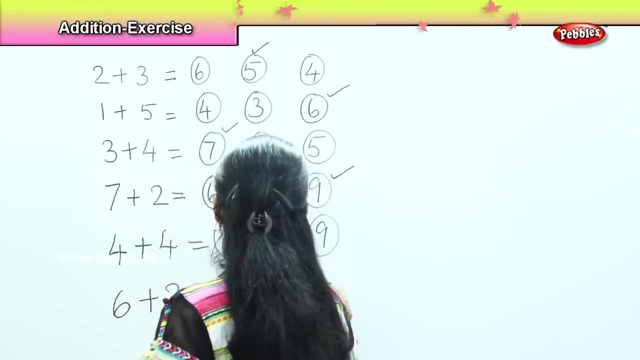 Shall, we count 1,, 2,, 3,, 4,, 5,, 6,, 7,, 8.. So what is my answer? My answer is 8.. The next question: 6 plus 3 is equals to what? So you need to again find out the answer for this question. 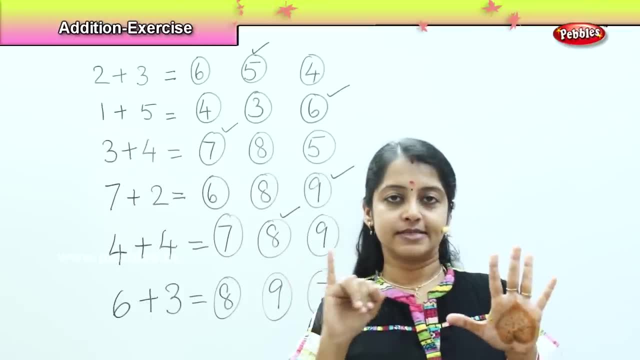 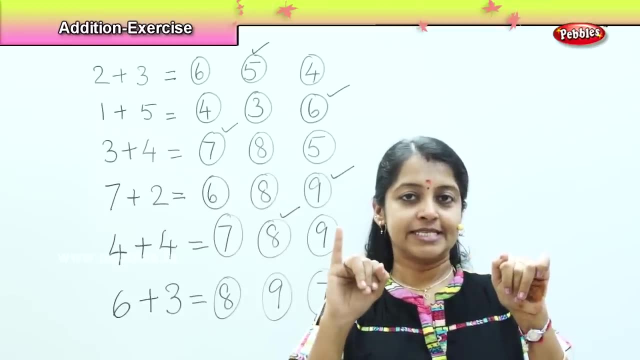 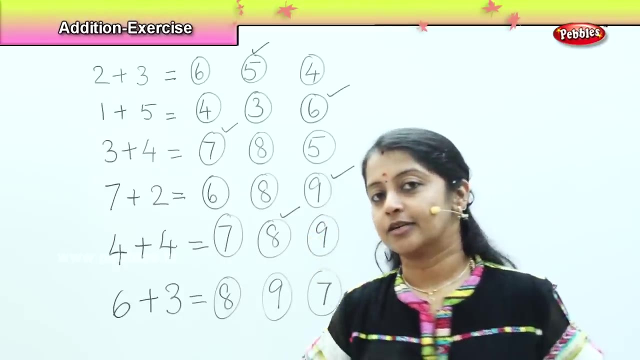 So what we need to do? We need to keep 6 fingers in the hand. Shall we count 1,, 2,, 3,, 4,, 5, 6.. add how many? 3.. So 7,, 8,, 9.. So what is my answer? The answer is 9.. So was it useful? 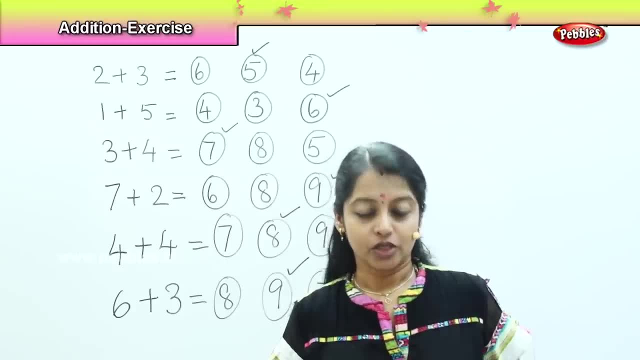 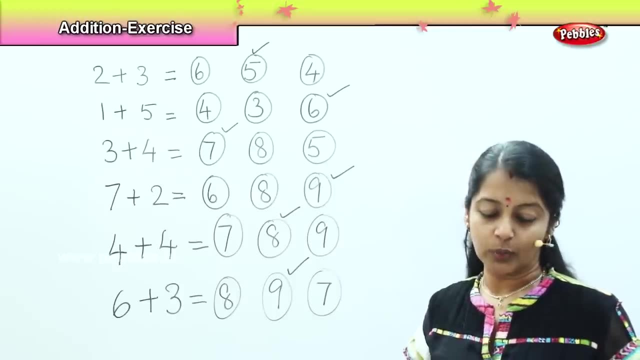 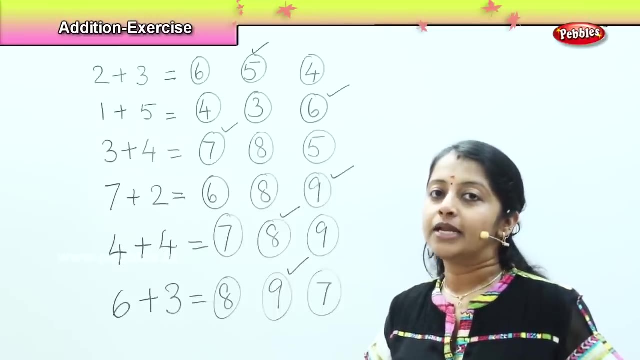 for you children. It was very easy, right. So now I will be giving you the next revision for the addition facts, what we learnt. Now I will be giving you a few numbers and you need to find me the addition fact for that particular number. So now we are going to. 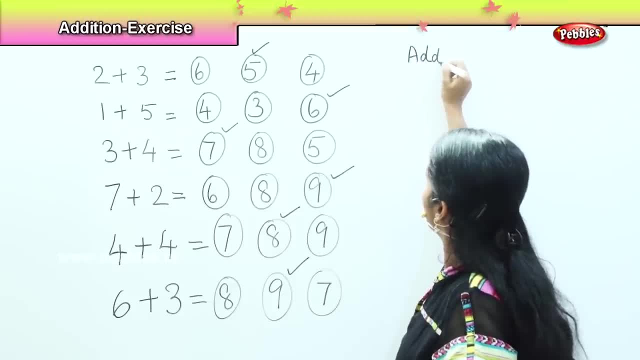 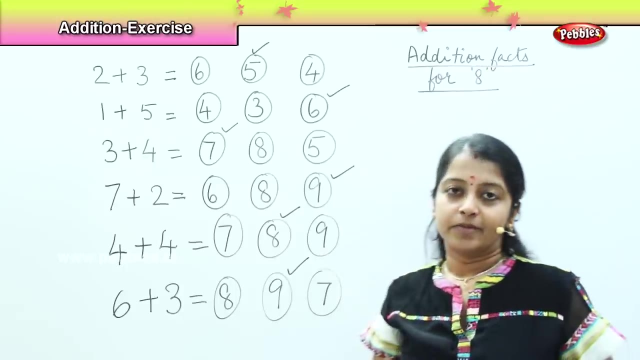 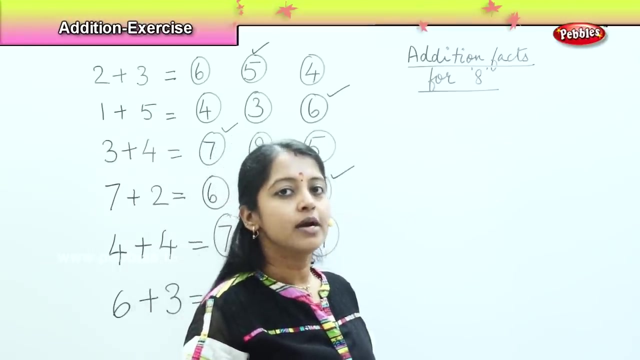 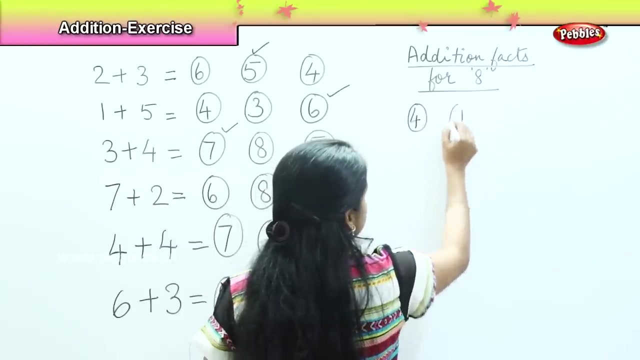 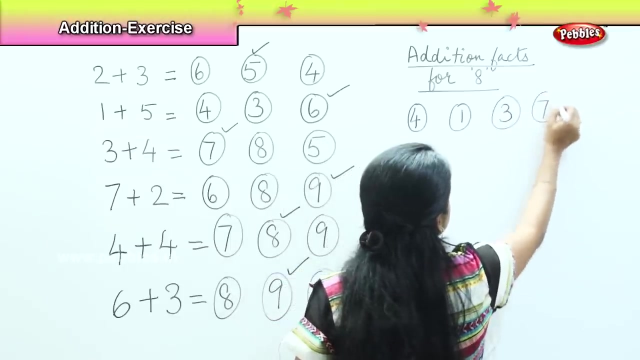 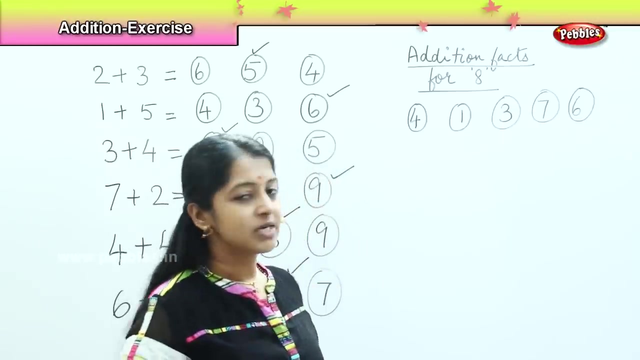 find the addition fact for number 8.. I will be giving you 4 numbers and whichever number will make the addition fact for 8. You need to colour that number. So the first question is: I have 4,, 1,, 3,, 7,, 6.. So what? 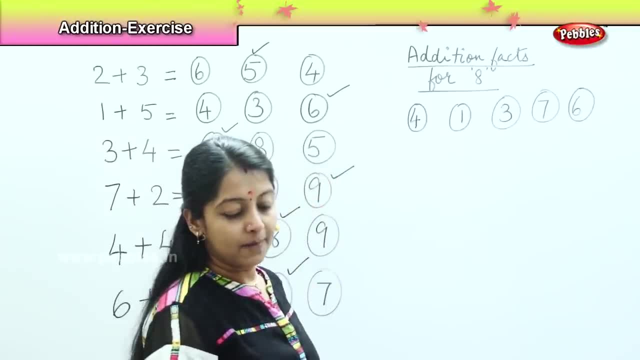 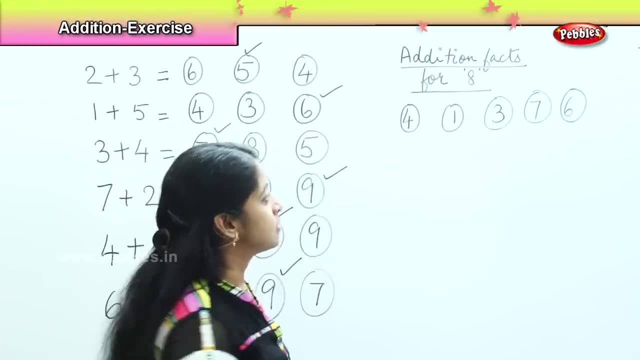 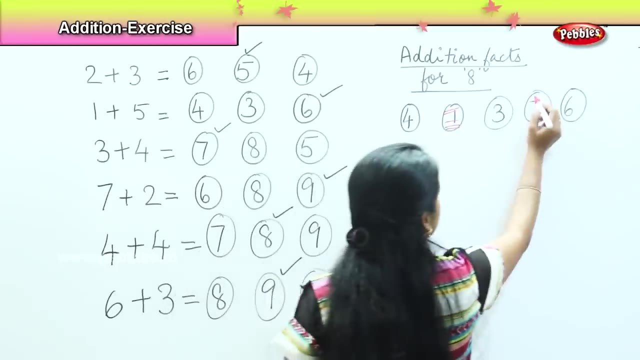 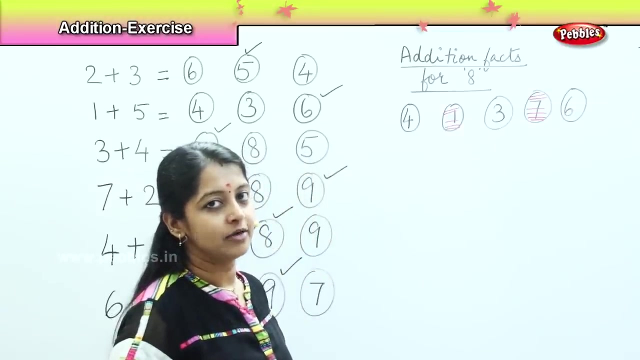 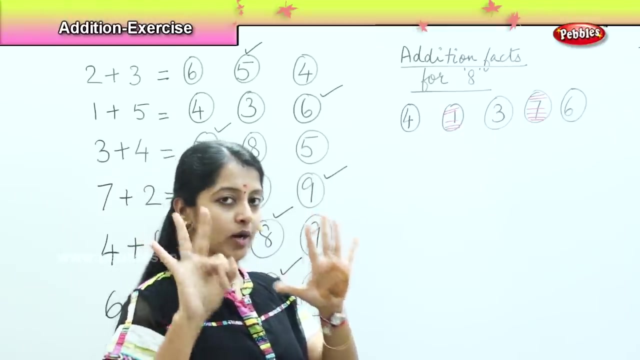 is the addition fact children Here. what numbers if I add, will I get the number 8? Yes, So if I select number 1 and number 7, I will get the addition fact of number 8.. So shall we try adding with the fingers? 7 when added with 1 will give me the answer 8. Is 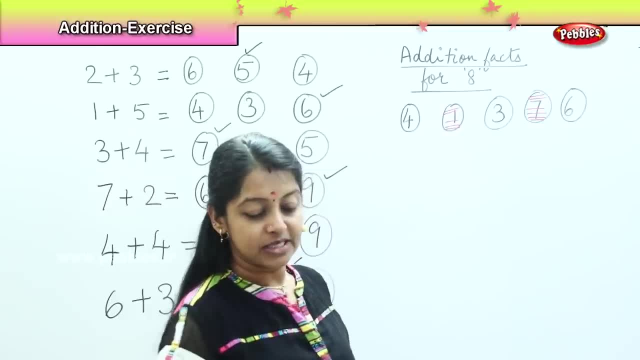 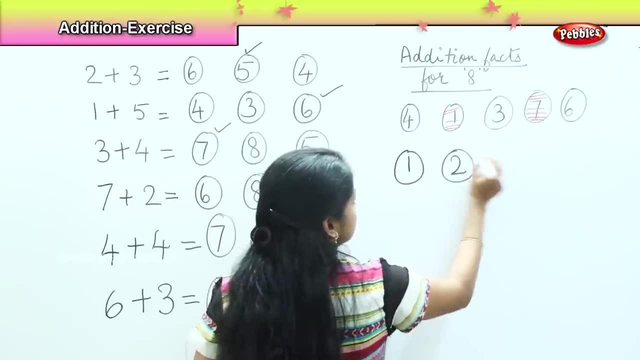 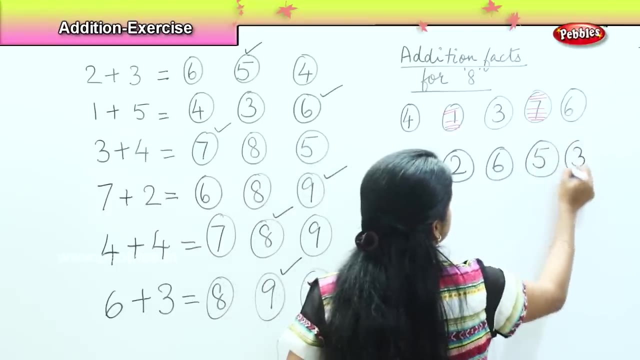 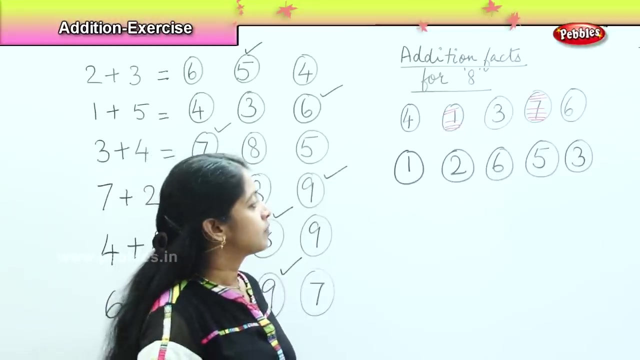 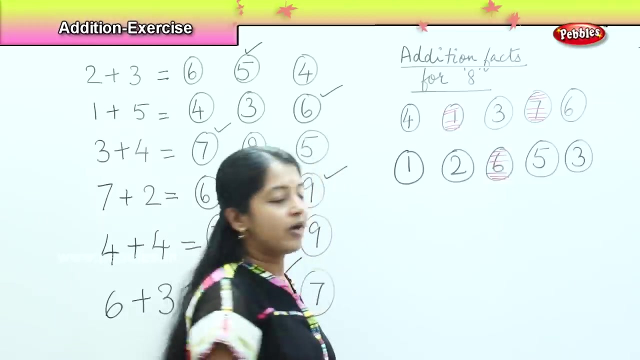 it correct? Yes, it is. Shall we try with the next question? So now, what is the addition fact? How can we frame number 8 here? So when I select number 6, what you have to add to 6 to make it correct. 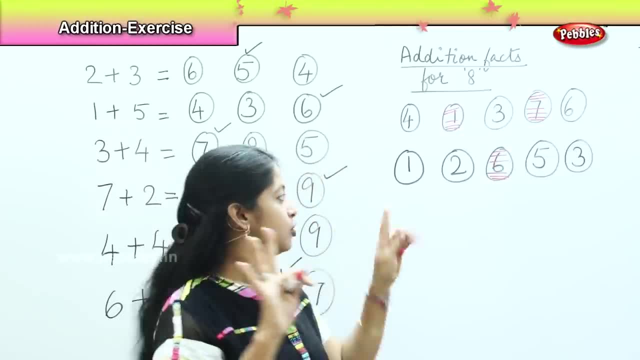 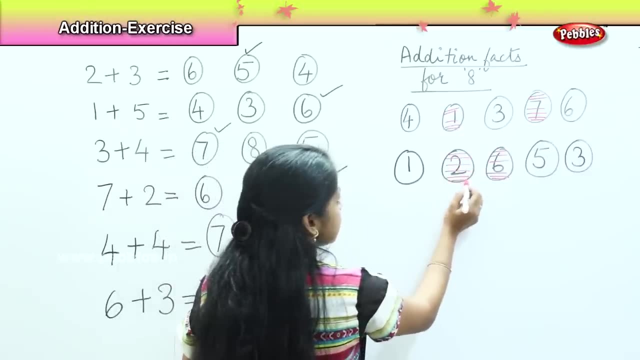 8,, 7 and 8.. So what is the next number which you will colour Very good, it is number 2.. So 6, when added with 2, will give me the number 8.. So is there any other number which will? 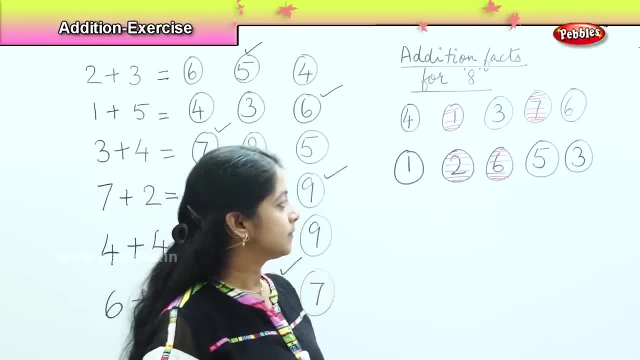 form number 8: children. Just see and tell: Yes, there is one more number. right, If I have 5 fingers in one hand and I add 3 more, What will it be? 4, 5, 6, 7, 8.. Do I get the answer Yes, So what will I do? I will. 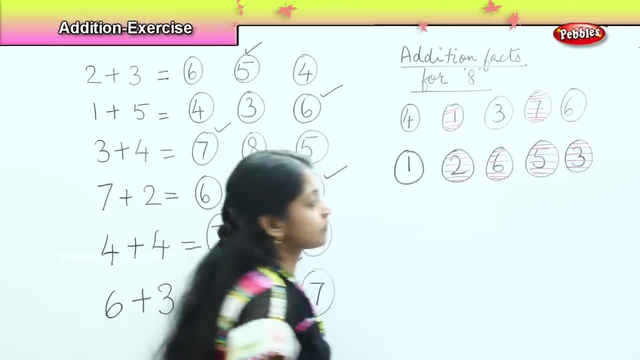 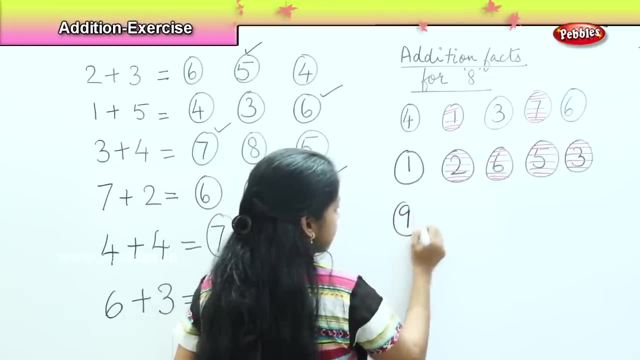 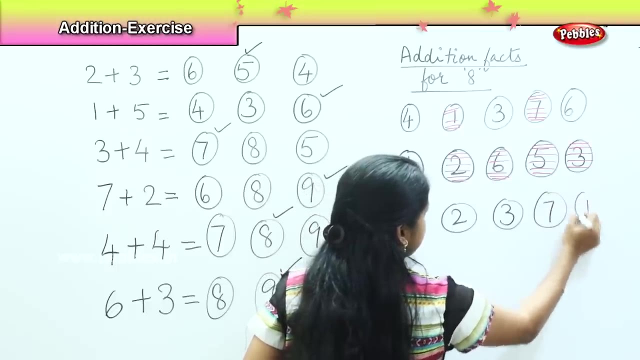 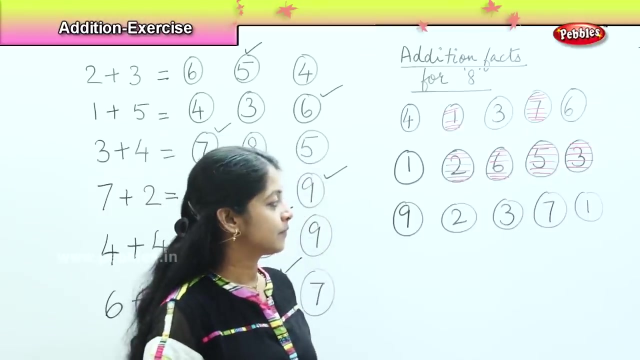 shade this number 5 and number 3 also. Yes, So one more question for you. So what is the addition fact here? children 8. 8. what is the addition fact? very good, you need to shade number 7 and number. 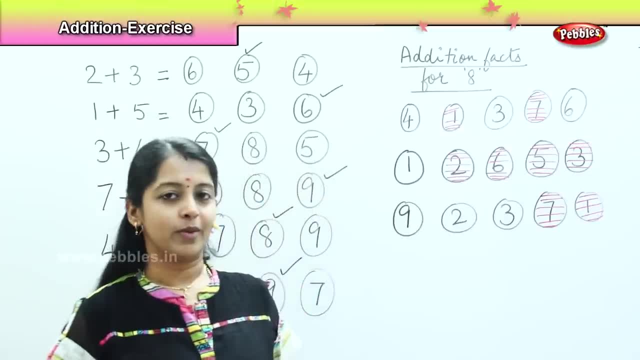 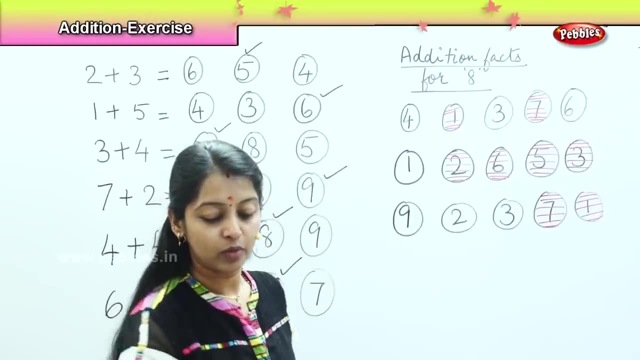 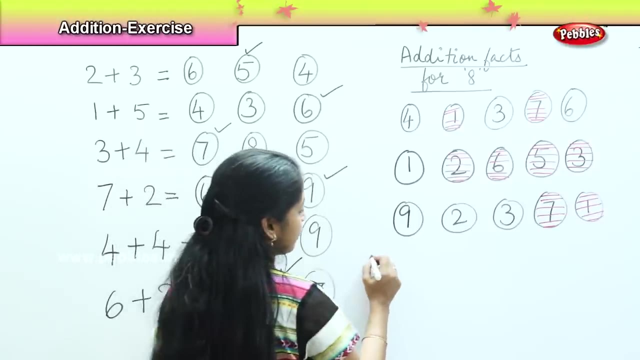 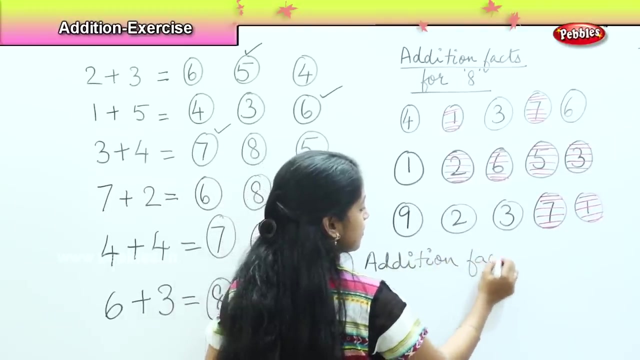 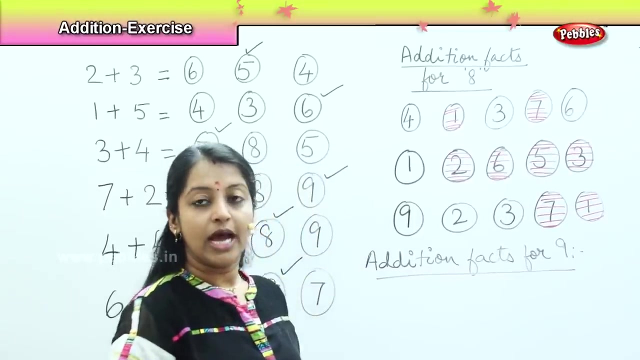 1. so 7 plus 1 will make number 8. so was it interesting. shall i give you the question for number 9? shall we do it? okay? so the next one is: you need to find the addition facts for number 9. okay, so i will give you your questions here. 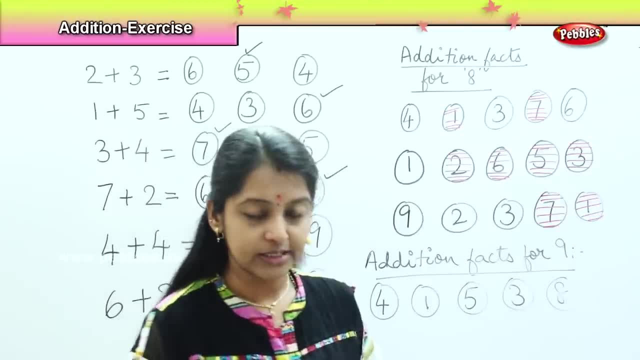 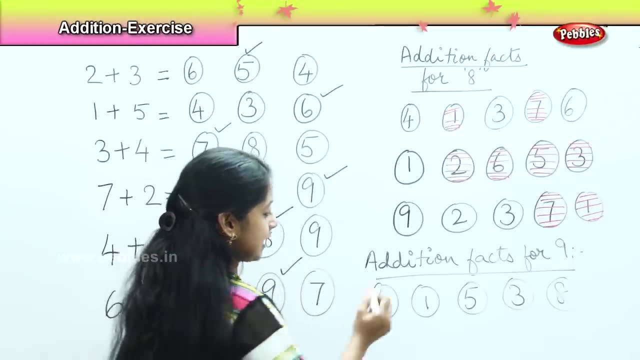 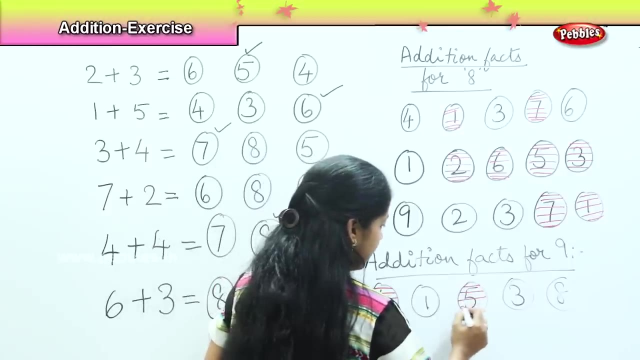 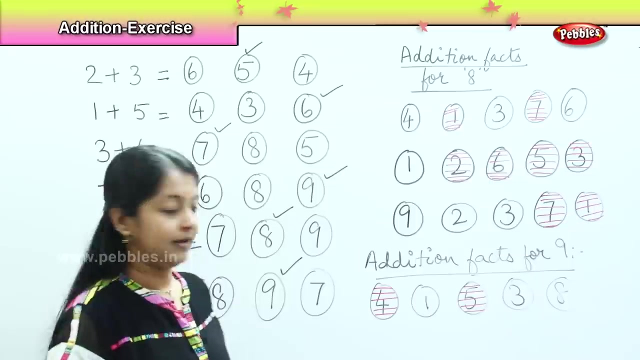 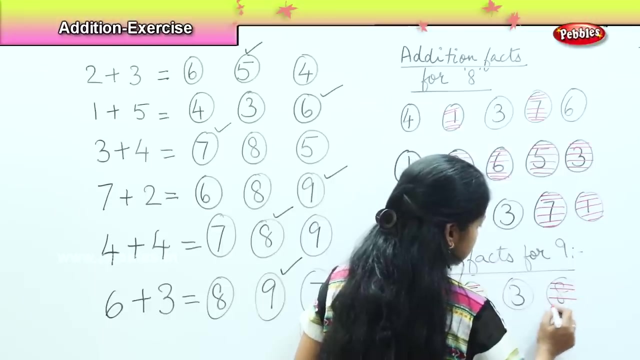 so which numbers if you select will give you the answer: 9. just see the board and tell me 9. very good, if i select number 4 and add it with number 5, i get number 9. is there any other addition fact? yes, if i add 1 and 8, i get 9. so what are the addition facts here? 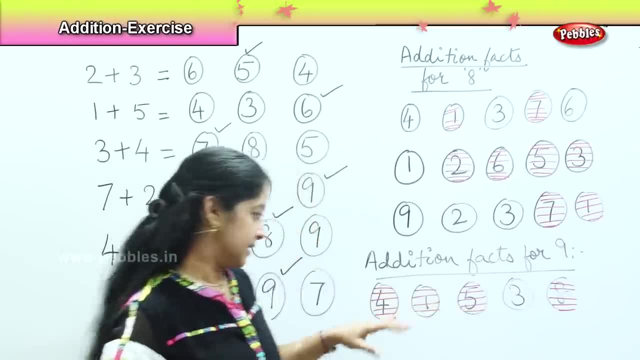 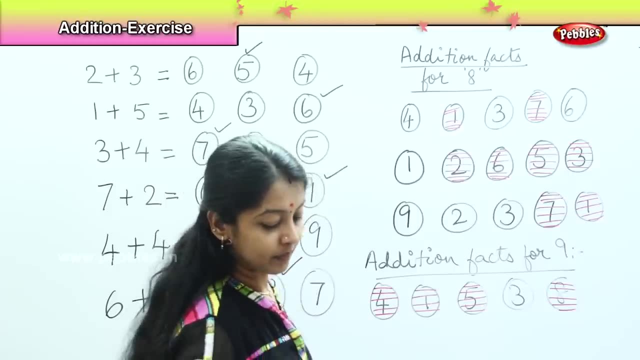 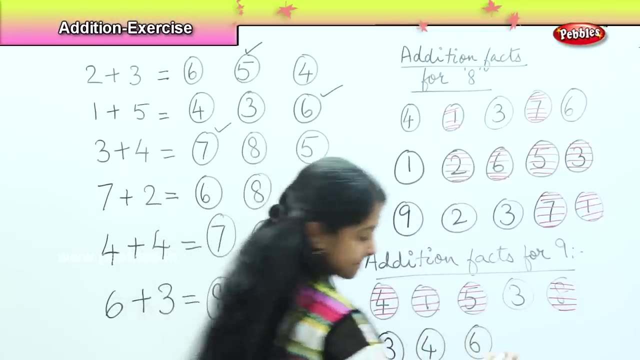 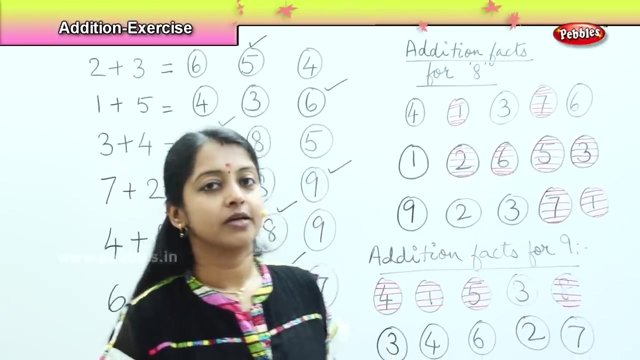 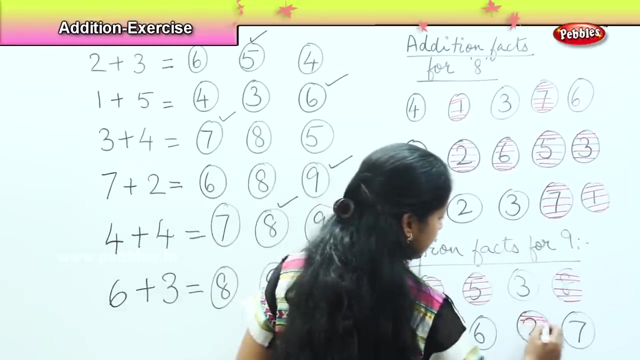 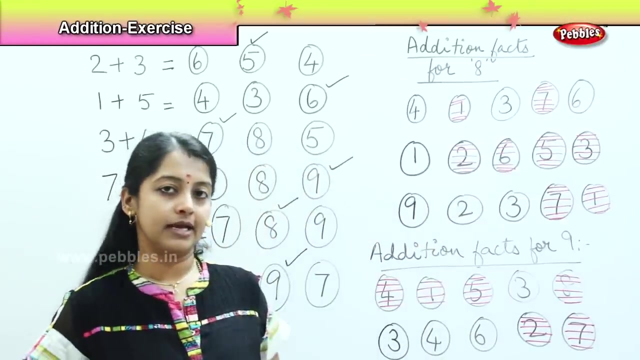 1 and 8 makes 9. similarly, 4 and 5 makes 9. shall we do with the next question? so what is the combination here? see the board and tell: very good, very good, very good. when I add 2 along with 7, it gives me the number 9.. Is there any other numbers in which we can make? 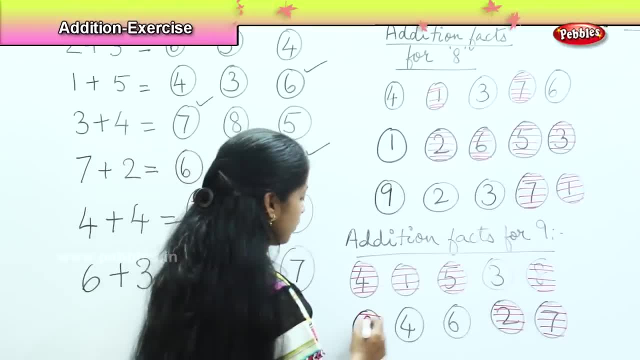 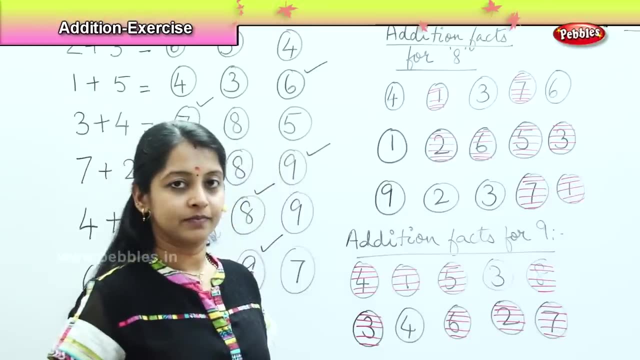 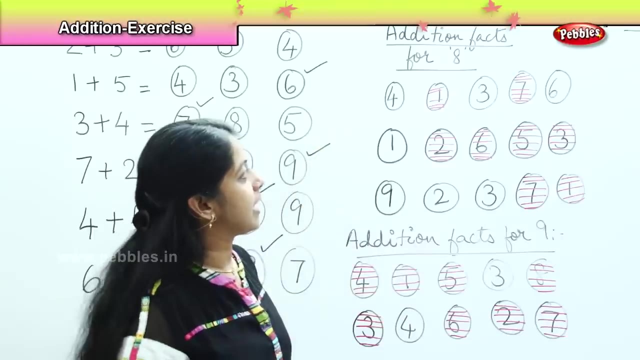 9?? Yes, there is one more addition fact, that is 3 and 6.. Fine, so shall we do a quick recap of what we have learnt now? Yes, so for addition fact 8, what was the possibilities here? 1 and 7.. 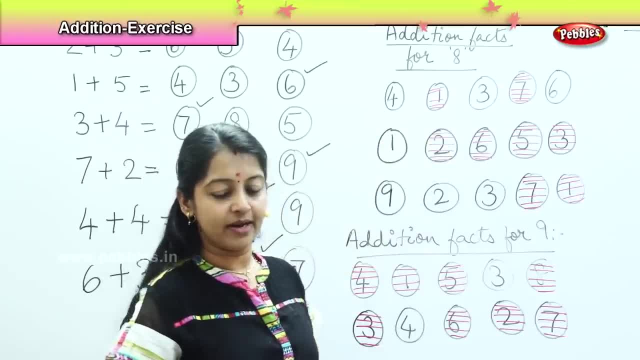 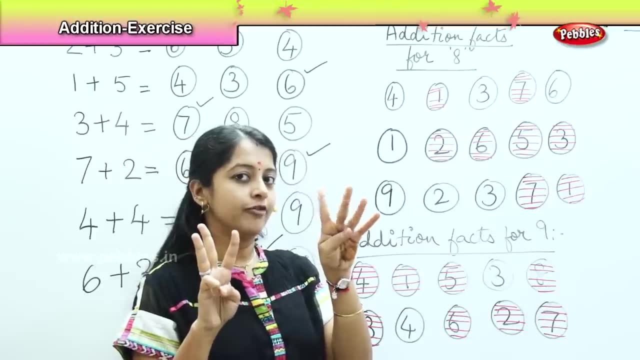 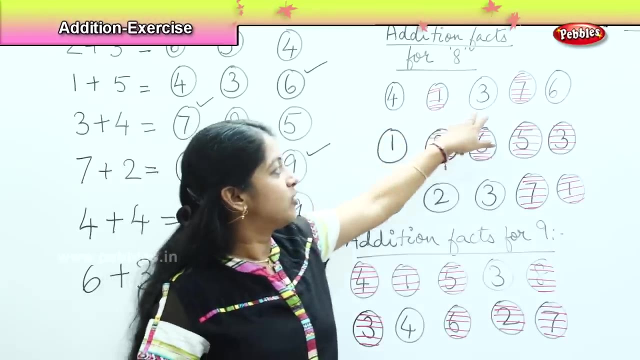 Why we could not add 4 and 3?. Shall we try Say: if I take 4 in hand and 3 in another hand, what is the total? I get 1, 2, 3, 4,, 5, 6 and 7.. But I want the answer number 8.. So 4 and 3 is 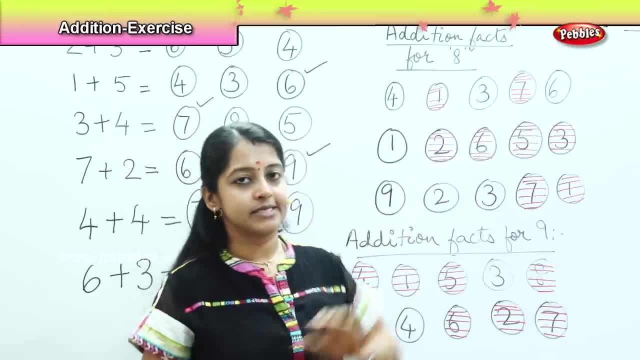 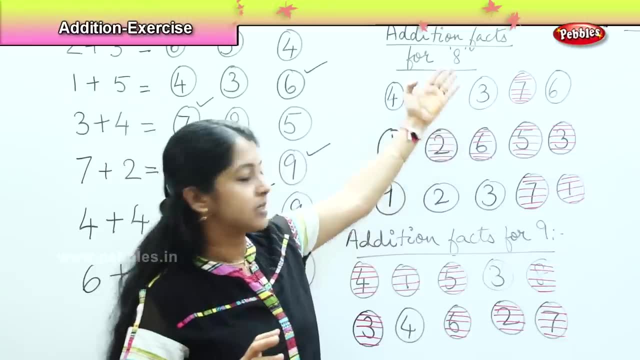 not possible. Now, if I take 4 and 3, what is the total? I get 1,, 2,, 3,, 4,, 5,, 6 and 7.. What if I take 3 and 6?? Say I take 6 fingers, then 7,, 8,, 9.. Again, my answer is not matching. 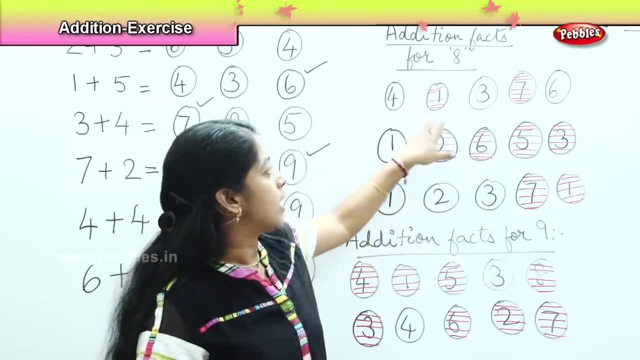 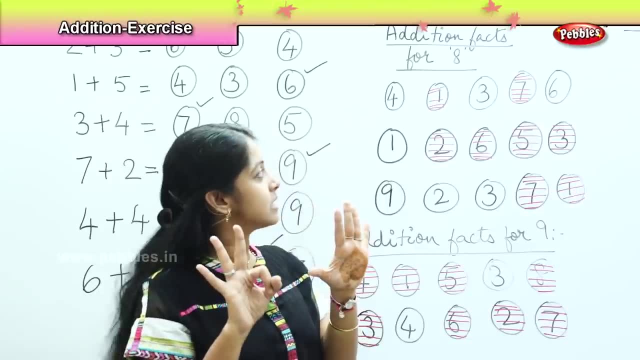 So there is only one possibility, which is 1 and 7.. Shall we try 7 fingers? when I add 1, it makes 8.. So is the answer correct? Yes. The next one: if I add 1 and 2,, 2 and 1,. 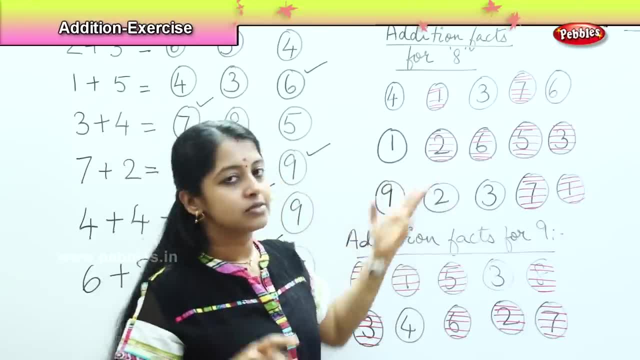 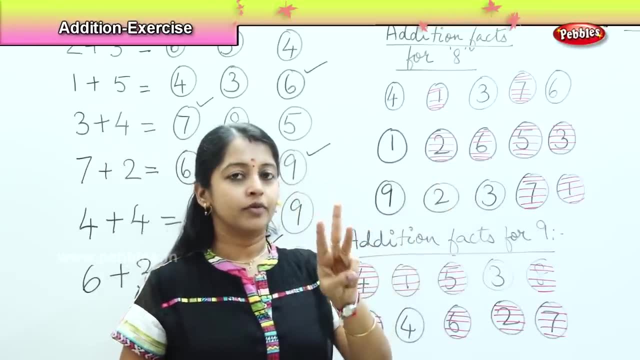 what is the answer? I get 3.. It does not solve my purpose If I take 2 and 6, say 2 in one hand, and then 3,, 4,, 5,, 6,, 7 and 8.. 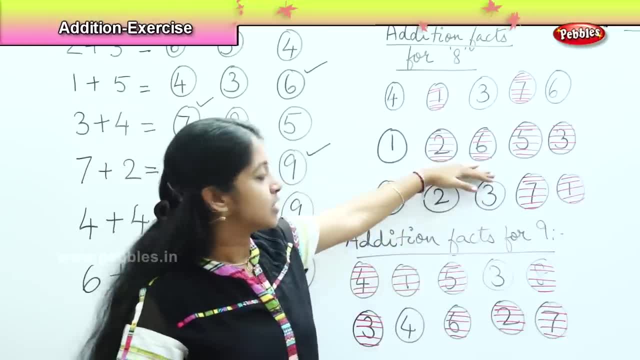 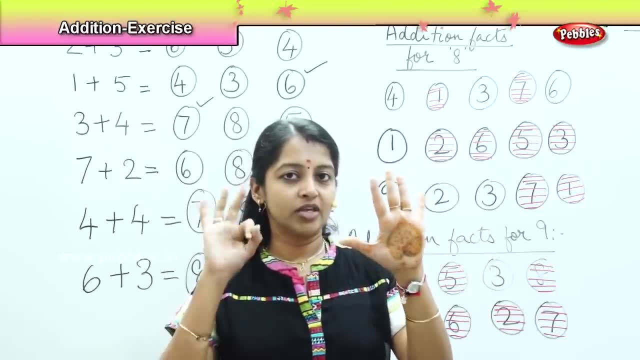 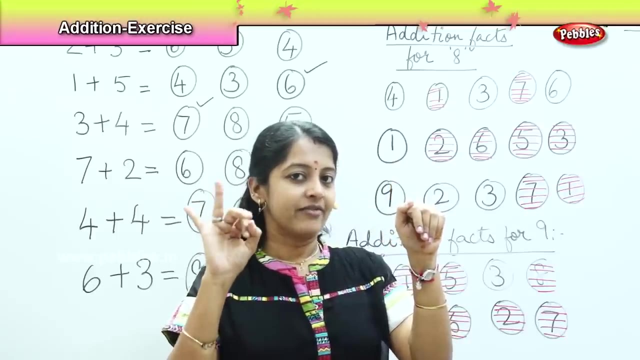 So am I getting the answer Yes. So 2 and 6 will make one possibility, And same thing 5 and 3.. If I take 5 fingers in one hand and 3, shall I count 1,, 2,, 3,, 4,, 5,, 6,, 7,, 8.. 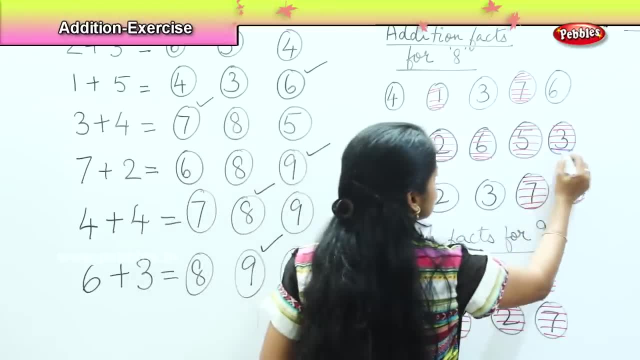 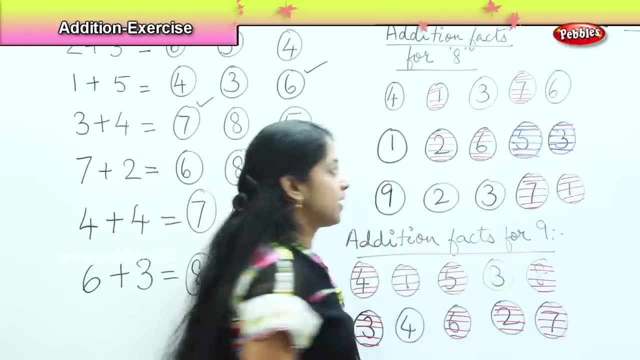 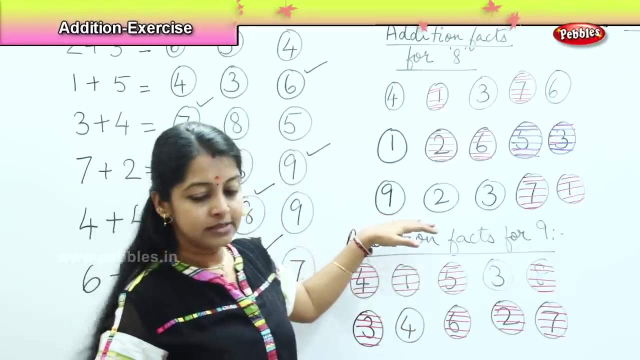 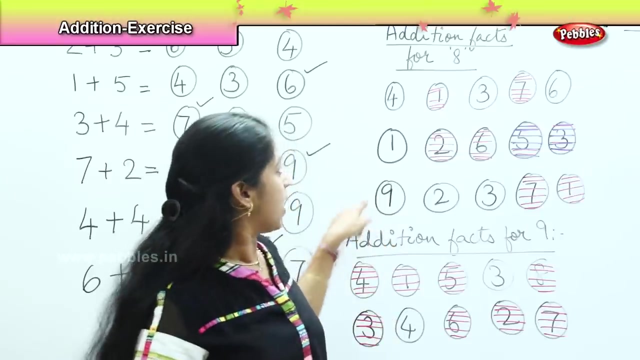 So do I get the answer? Yes, So the two possibilities are 2 and 6 and 5 and 3.. Right, there are two possibilities here. In the next question again see: 9 is there. If I have 9 fingers and I add 2 more, it is 10 and 11.. But I need the answer 8.. So it does not match. 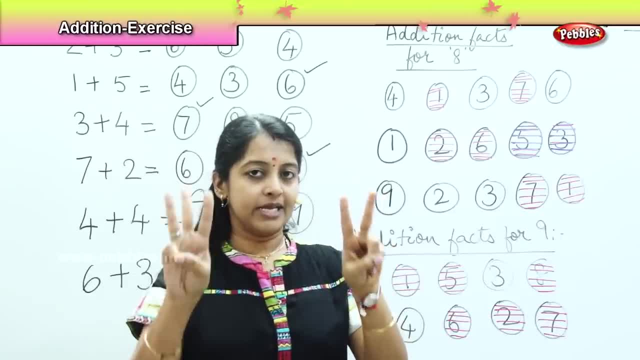 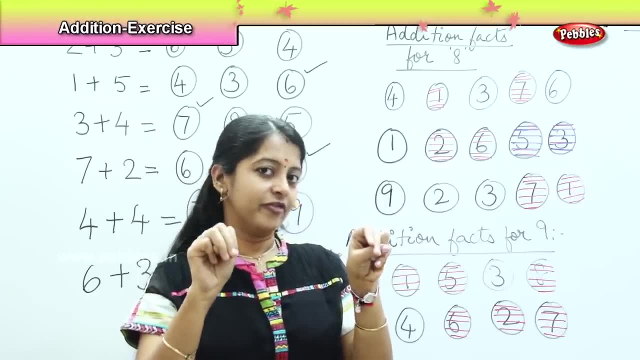 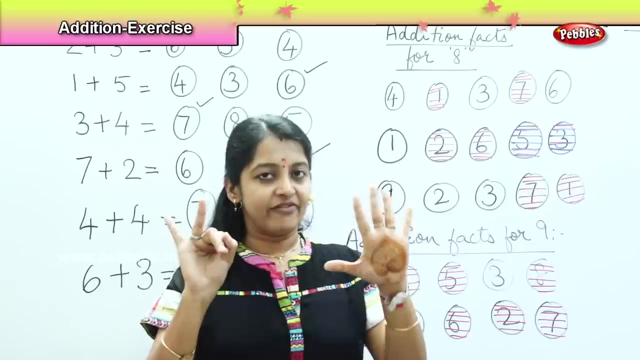 If I add 2 and 3, I keep 2 fingers and I keep 3 fingers. If I add 2 together, what is my number? 1,, 2,, 3,, 4, 5.. Again, this does not solve my purpose. Now, if I add here 7 plus 1, does it solve? Yes, 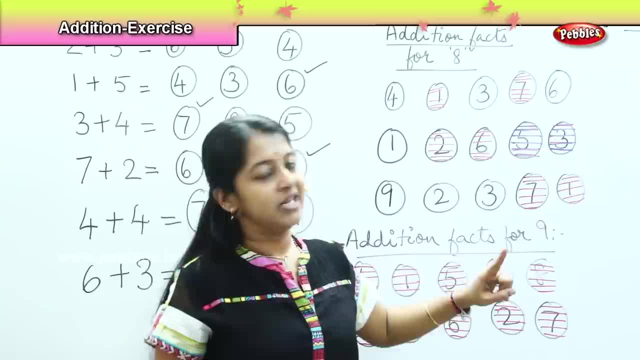 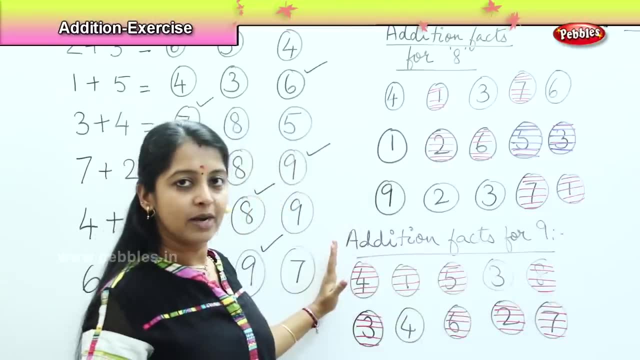 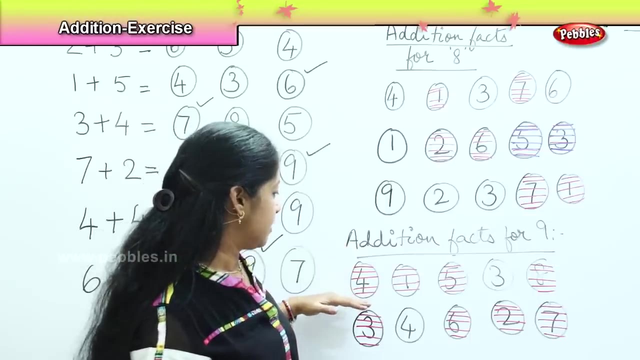 So here I have only one combination, which is 7 and 1.. Clear children: Yes. So shall we do it for number 9?? Shall we check Whatever answer we have selected is correct or not? Ok, fine, I have selected 4 and 5.. Right, I keep 4 in one hand and 5 in one hand. 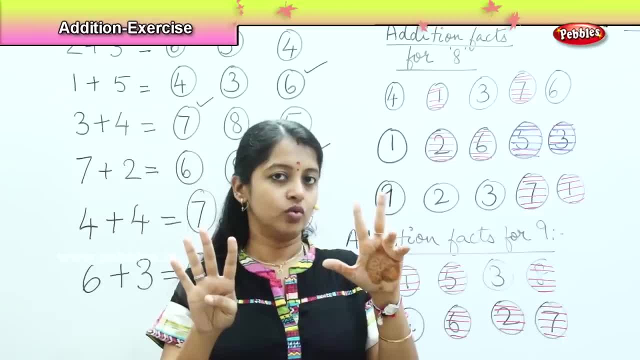 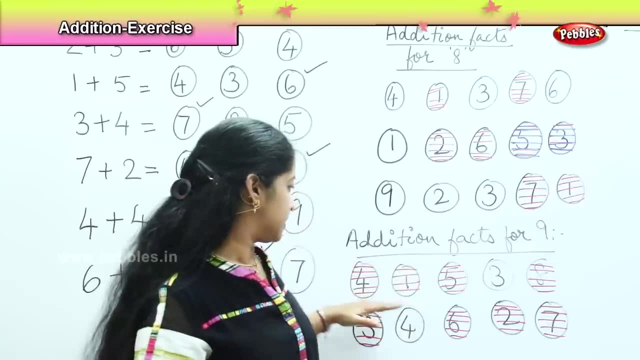 What is the total? I get 1,, 2,, 3,, 4,, 5,, 6,, 7,, 8, 9.. So is it matching here? Yes, What is the next possibility? you selected 1 and 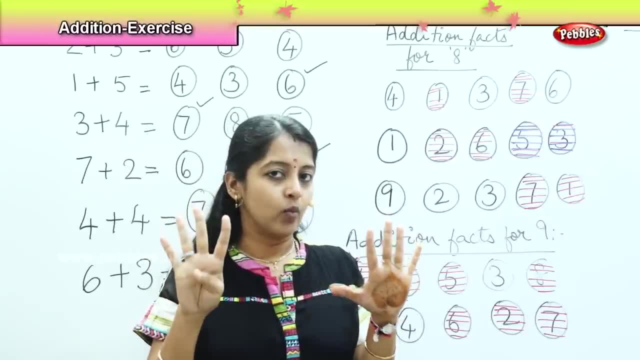 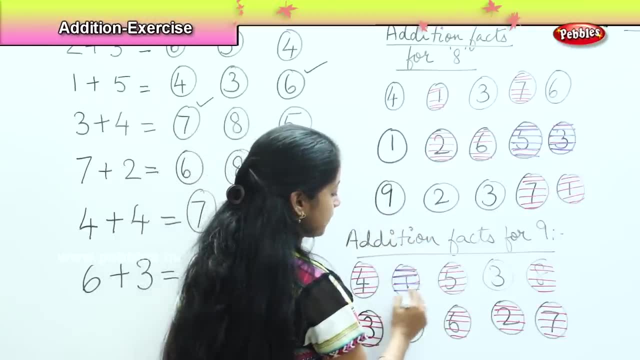 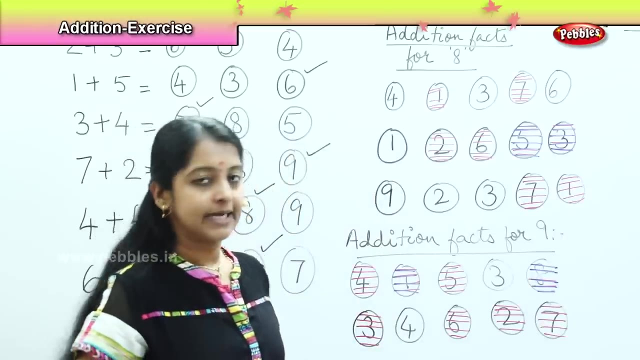 8.. I keep 8 fingers and then when I add 1 more, it becomes 9.. So the second possibility is 1 and 8.. So is it correct? Yes, The option is correct. Coming to the second one, If I add 3 with 4, does it make an answer? Just try. 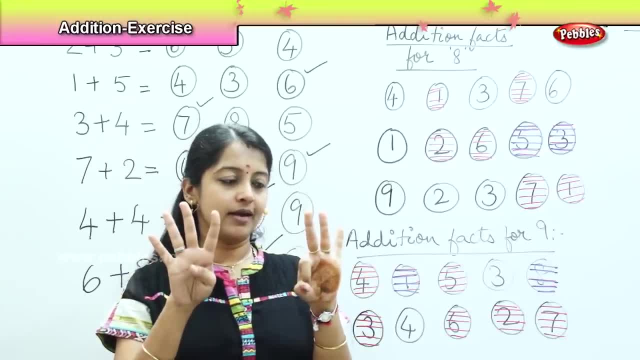 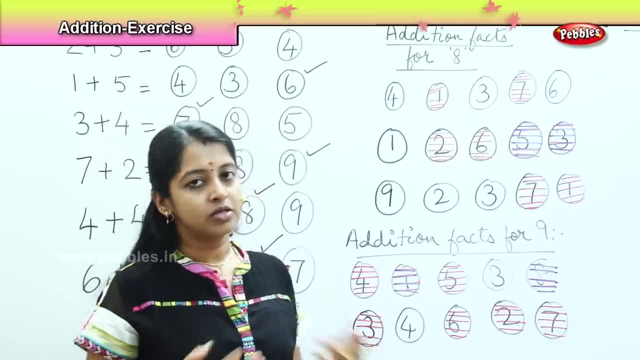 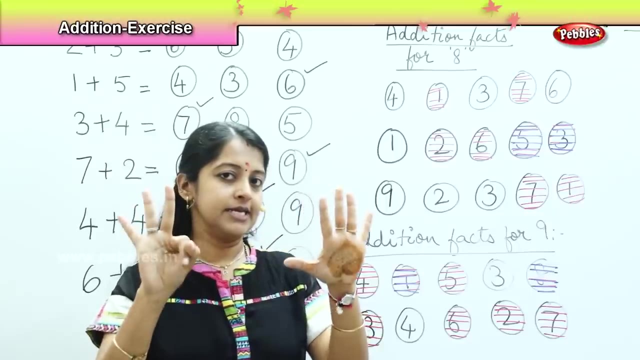 3 in one hand, 4 in one hand. What is the total? I get 2,, 4,, 5,, 6,, 7.. So it does not solve my purpose. If I add 3 with 6, does it solve 6,, 7,, 8,, 9.. 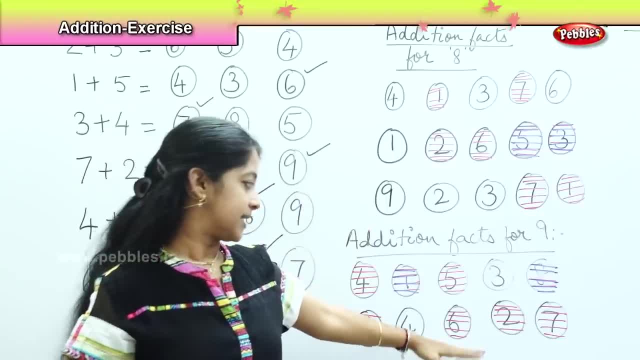 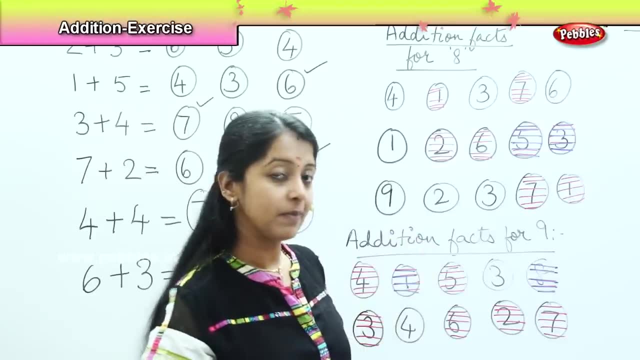 So my first combination is 3 and 6.. If I add 2 and 7,, 7,, 8,, 9.. So does it solve my purpose? Yes, So what are the two different options here? Here it is 3 and 6.. 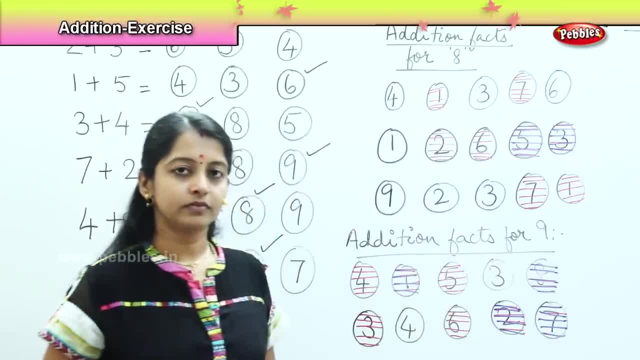 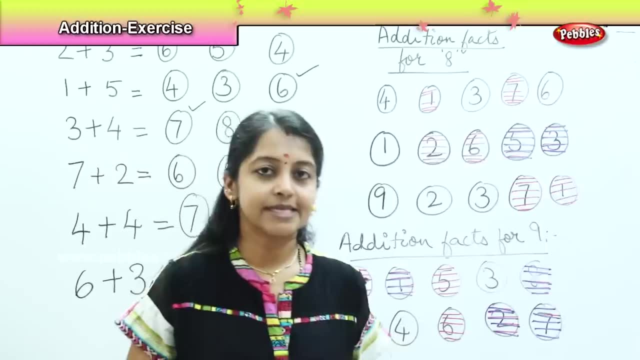 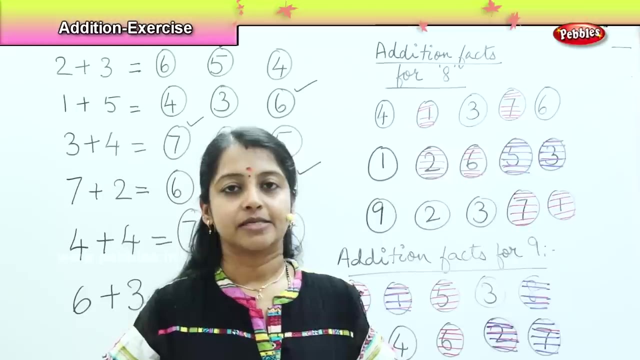 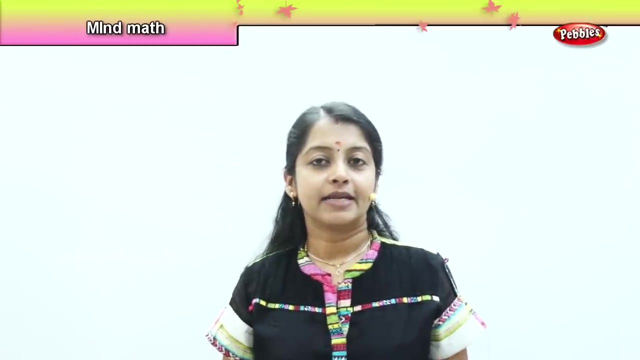 and 7 and 2.. So, children, I hope all the methods are very clear with you and you have enjoyed doing all the exercises with me, Yes, so it was fun learning addition using different methods. So, children, after doing so many methods and techniques, in addition, we have 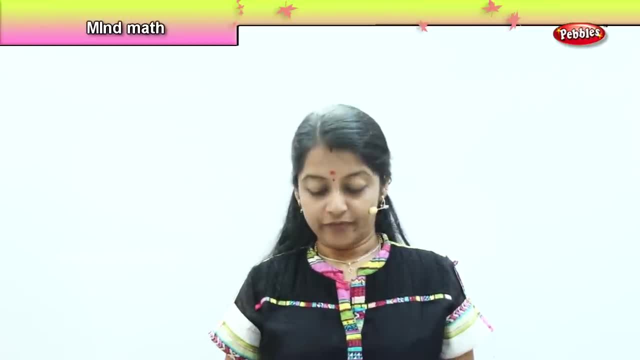 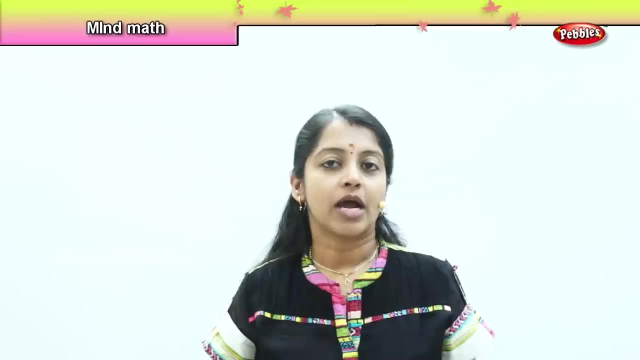 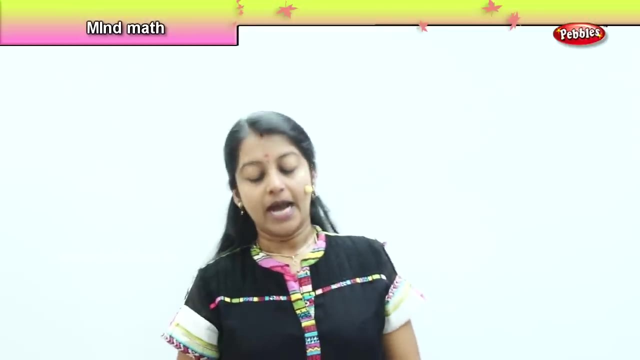 done a quick recap also, right? So now we are going to play a mind game. fine, I am going to ask you few questions and you need to answer me those questions. So shall we start? Yes, Now, Akhilan has got 4 pencils with him. How many pencils He has got 4 pencils. 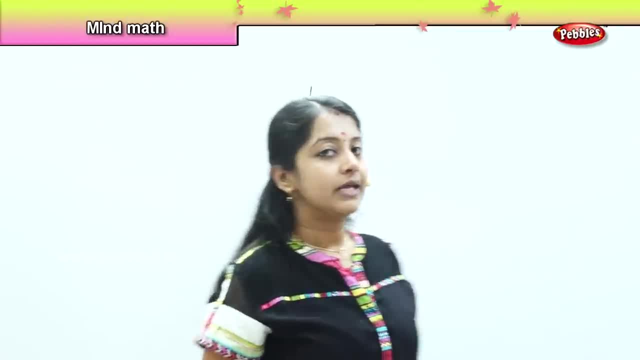 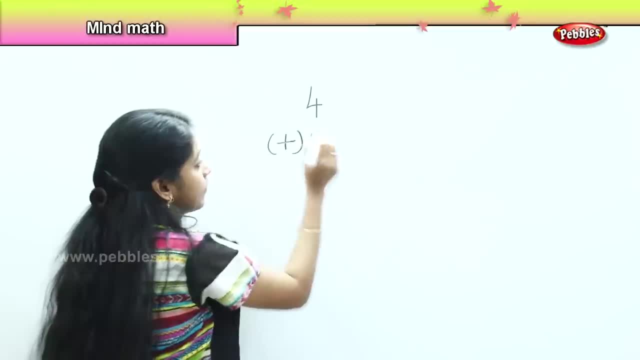 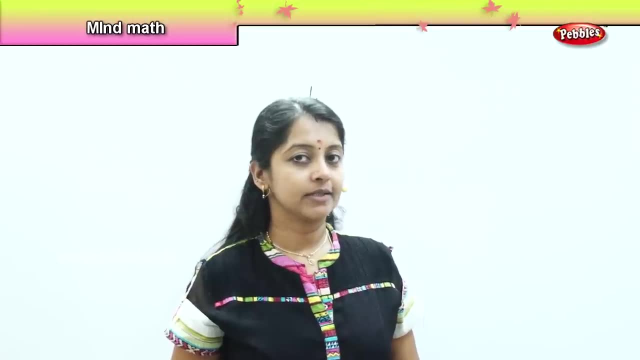 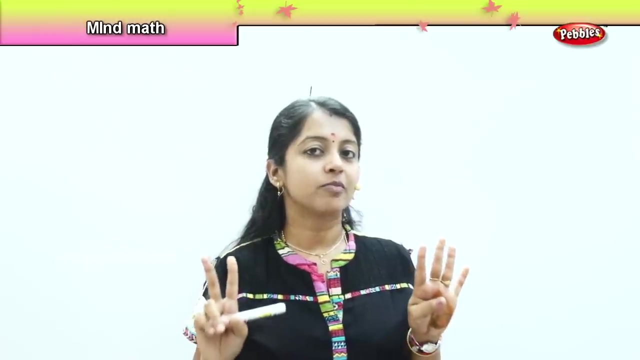 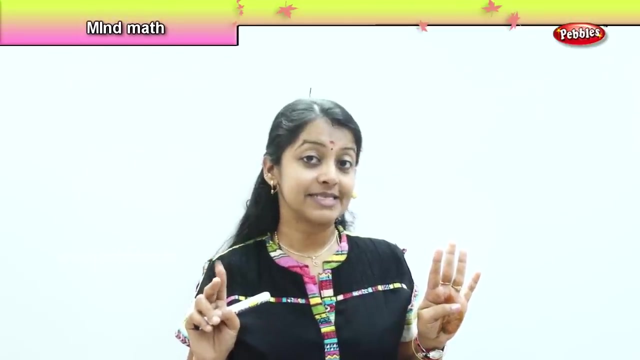 So he has got 2 more pencils. Okay, So what is the total number of pencils which Akhilan has? Can you answer me quickly? Akhilan has how many pencils? 4.. His friend, Mukhilan, gave him how much? 2.. So what is the total number of pencils? Akhilan has 1,, 2,, 3,, 4,, 5,, 6.. 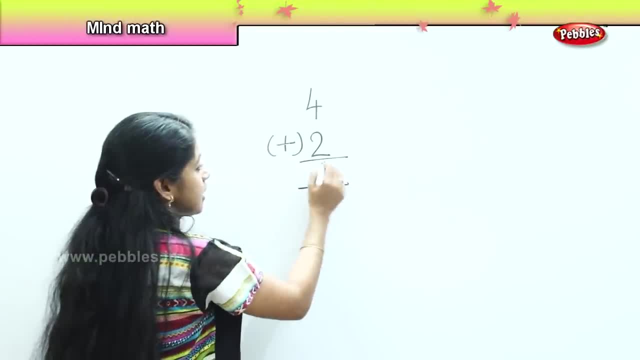 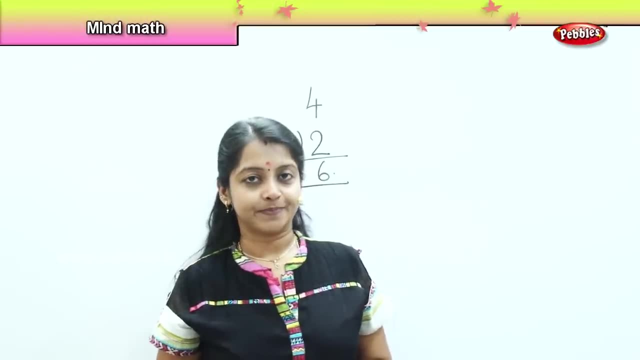 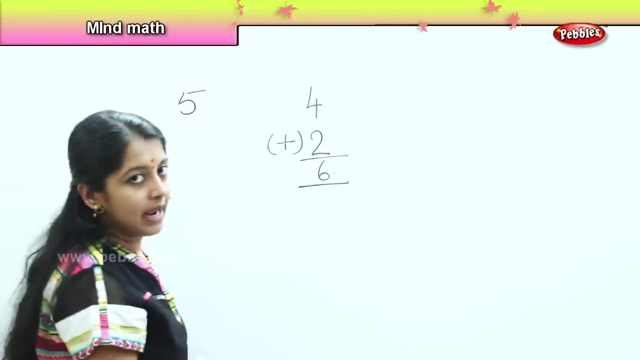 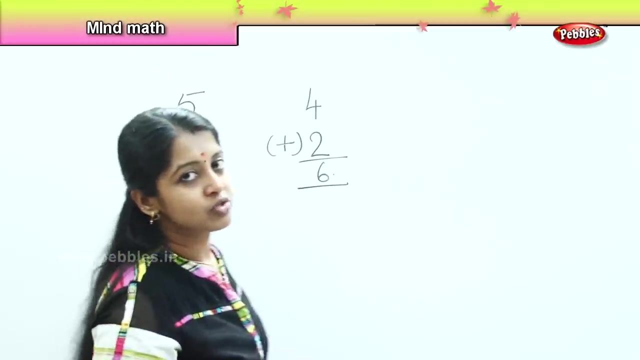 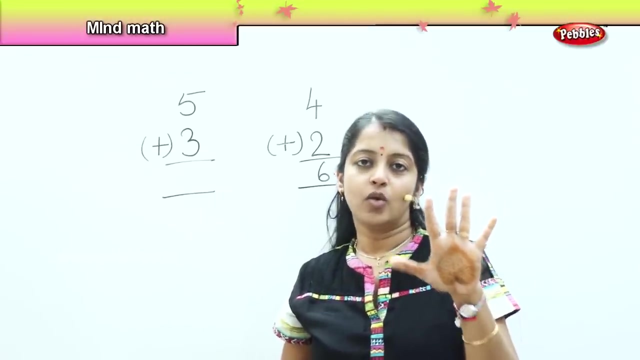 Very good. So the total number of pencils which Akhilan has is 6.. Okay, So I will give you another question. There are 5 flowers in one plant, Okay, And there are 3 flowers in another plant. So how many flowers do I have in total? So what did? 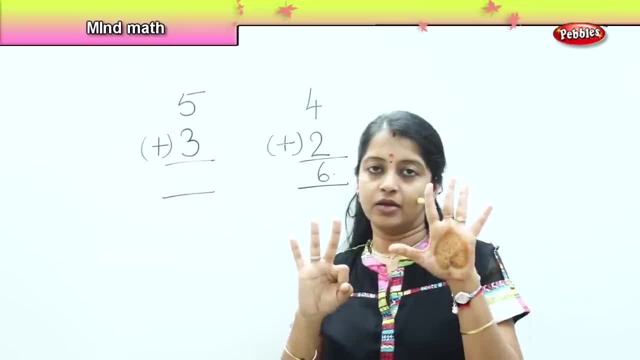 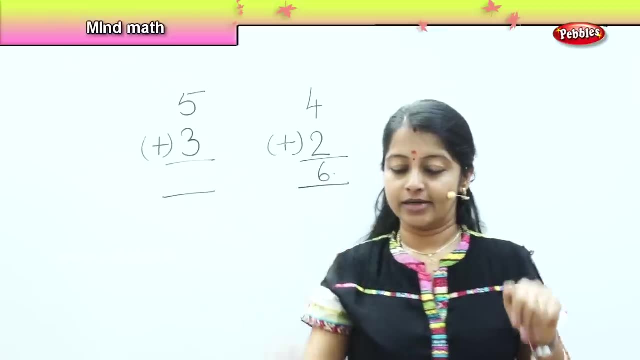 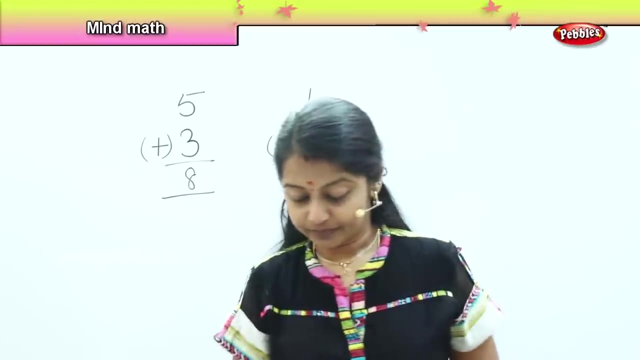 I say There are 3 flowers in another plant. So how many are there? 1,, 2,, 3,, 4,, 5,, 6,, 7, and 8.. So what is the total number of flowers I have? It is 8.. Very good Now. Ruby's father. 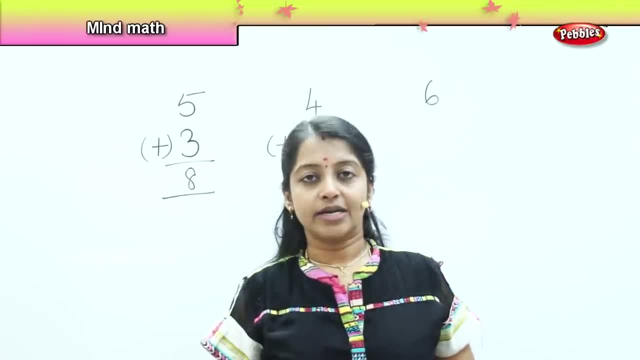 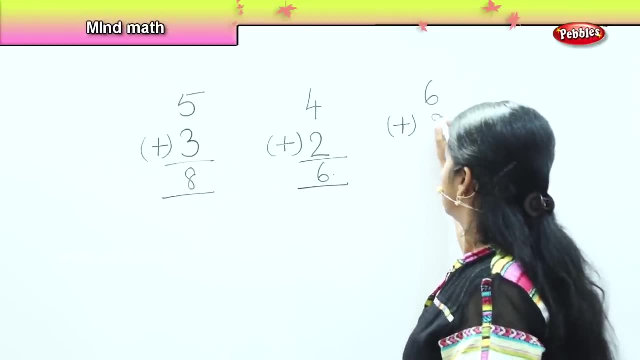 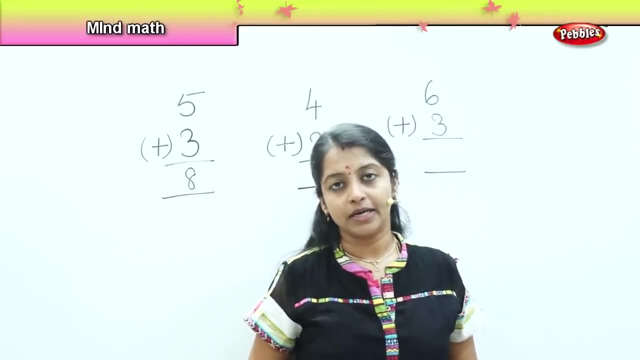 gave her 6 chocolates on her birthday. Okay. And her mother bought her 6 chocolates- Okay. Ruby's father bought her 3 more chocolates on her birthday. So what is the total number of chocolates which Ruby has on her birthday? Shall we count the number of chocolates? So